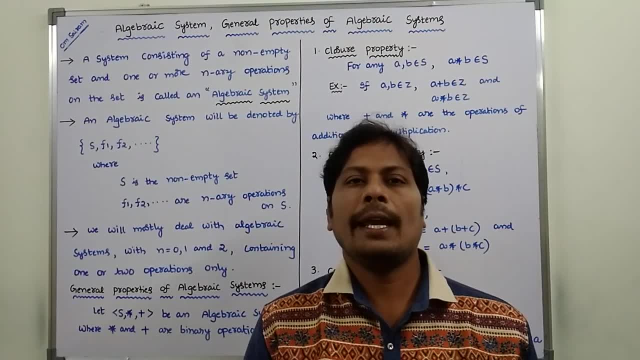 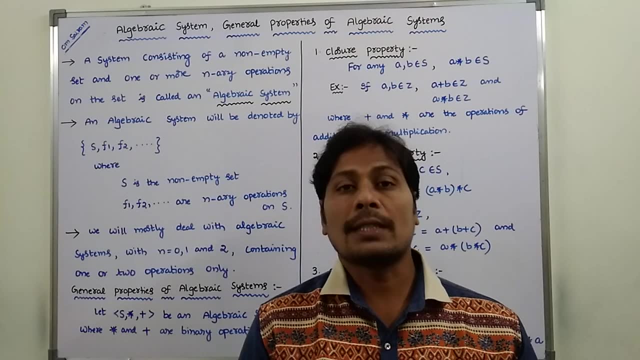 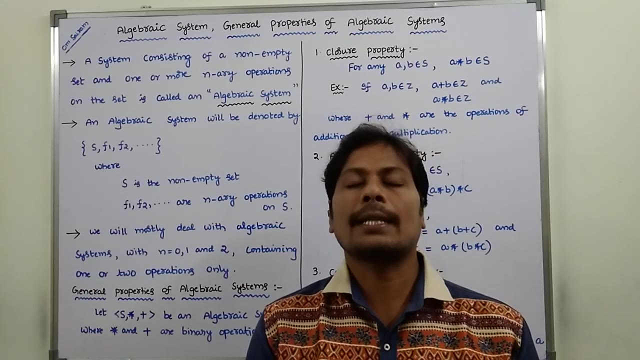 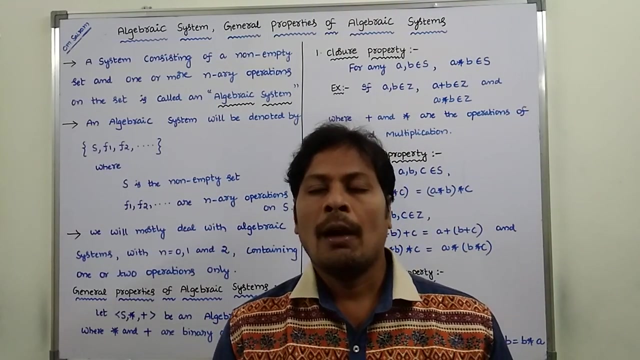 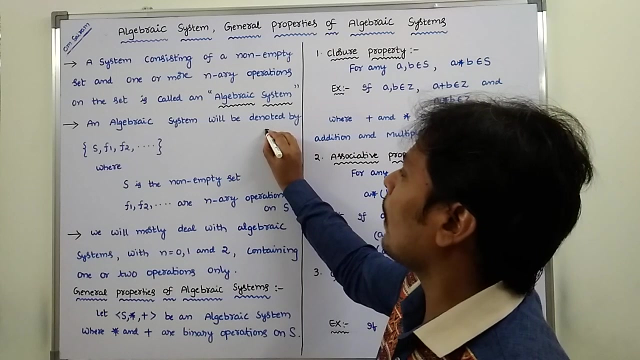 Hi, friends, today I am giving a lecture on what is algebraic system and what are the general properties of algebraic system. These are the points that we are discussing in this video. First of all, what is algebraic system? Algebraic system means a system consisting of a non-MT set. 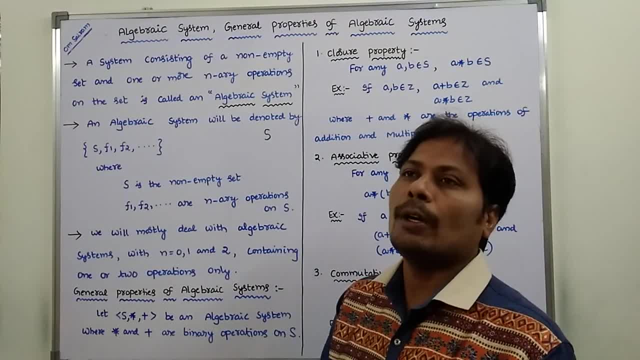 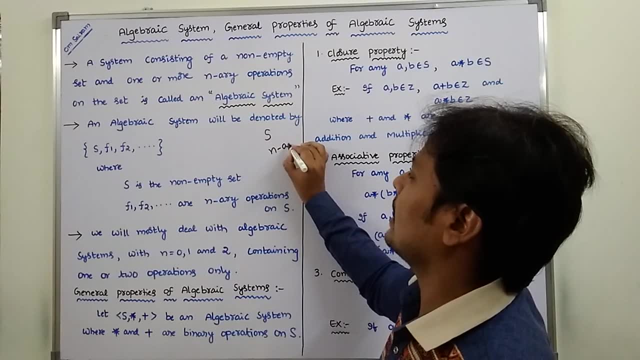 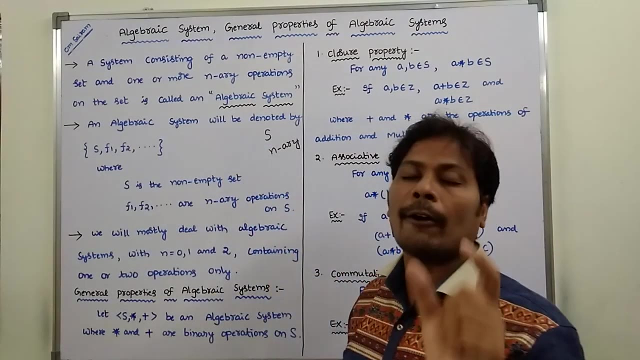 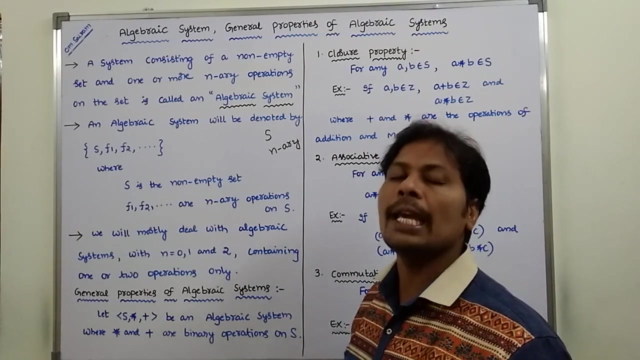 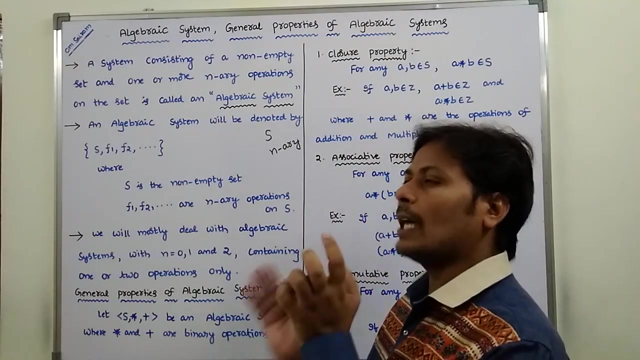 S on which N array operations are performed on the set. N array operations performed on the set. Here a system consisting of a non-MT set S on which non-MT set. we have to perform N number of operations on that set. So that is called as algebraic system, Generally algebraic. 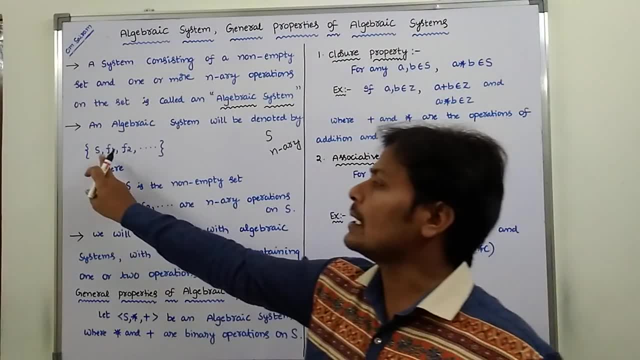 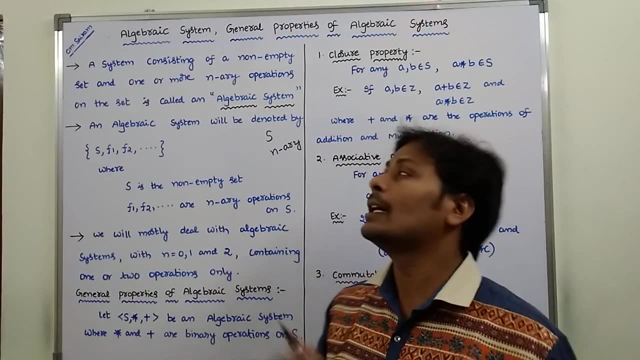 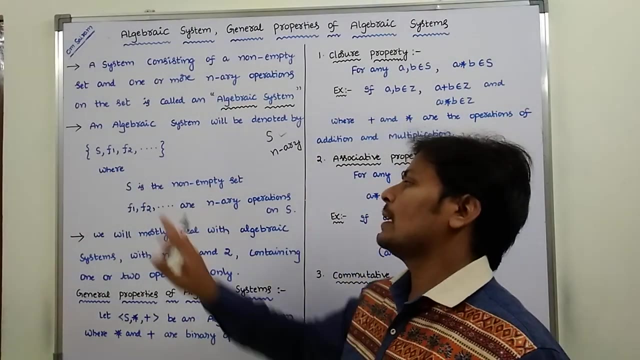 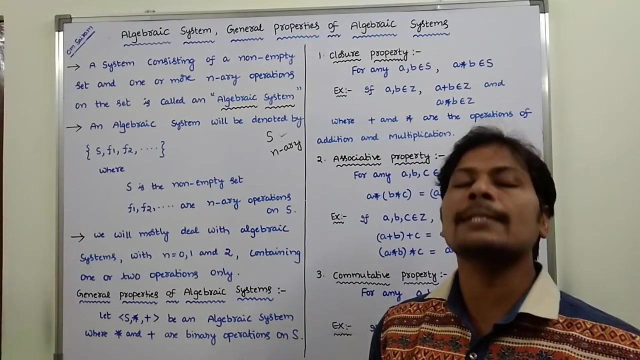 system can be represented by S, F1, F2, etc. Where S is nothing but non-MT set. Okay, so on that non-MT set, F1, F2, F3, F4, etc. are N array operations performed on the set. 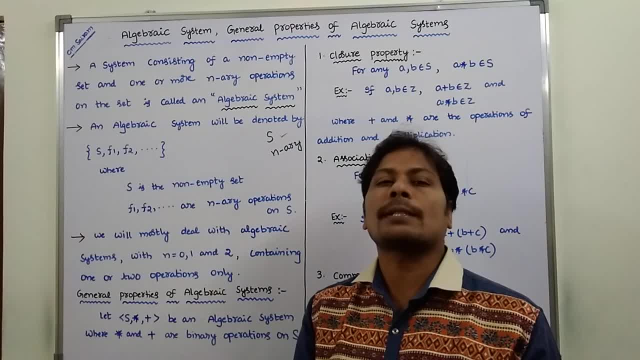 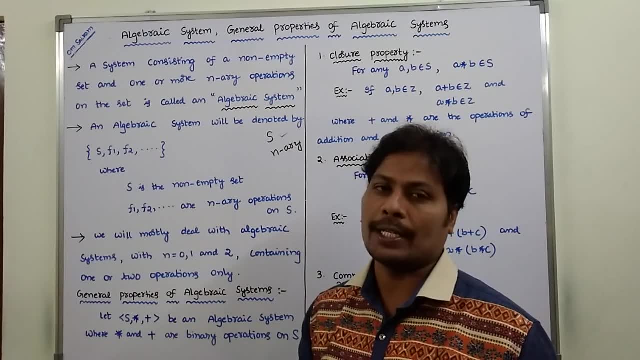 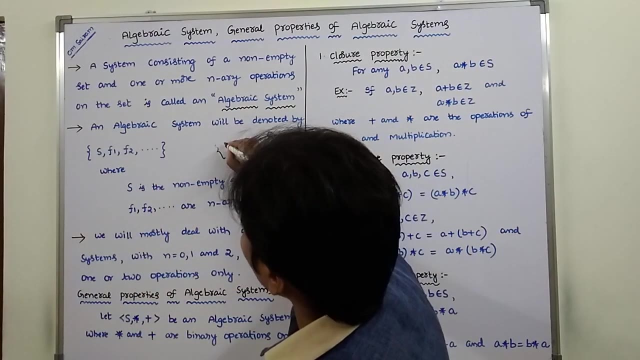 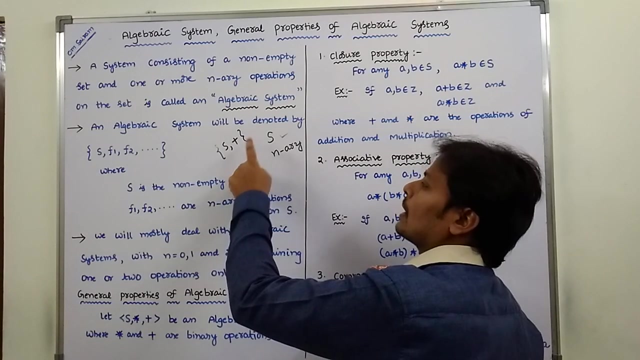 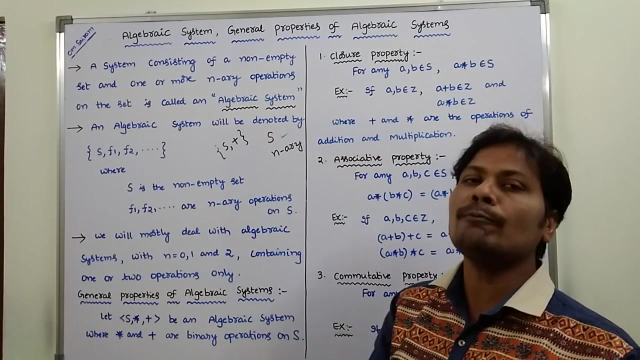 Generally, most algebraic systems which deal with N is equal to 0 and 1 and 2 operations, For example. so S, F1, F2, the system country, N is equal to 1 operator. okay, algebraic system with the sun yam. 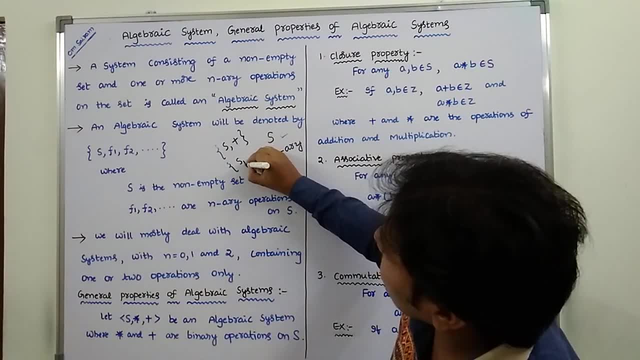 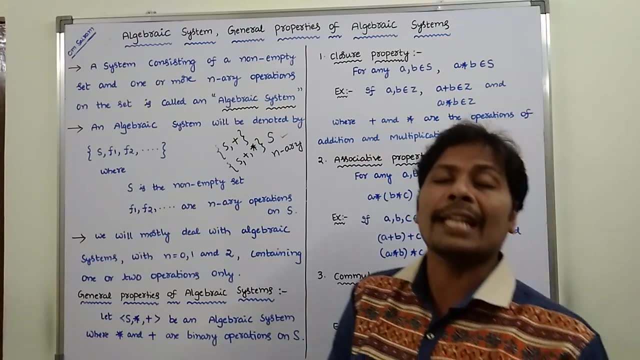 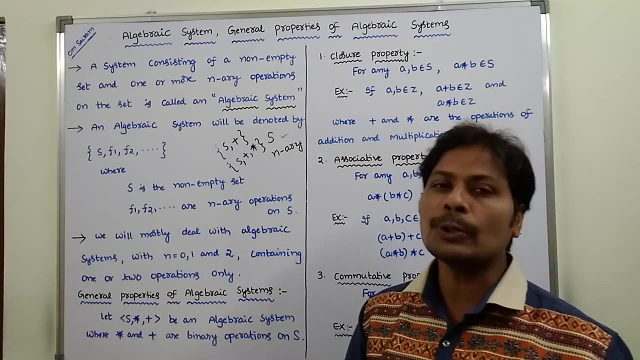 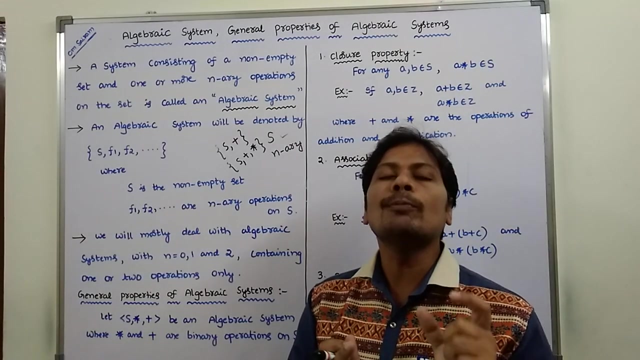 Okay, the second case: S comma plus comma e2.. Here the algebraic system which deal with two operations. Here n is equal to 1.. Here n is equal to 2.. Most of the algebraic systems which deal with one or two operations. 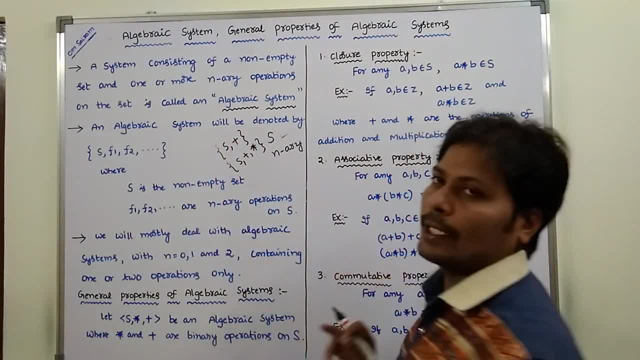 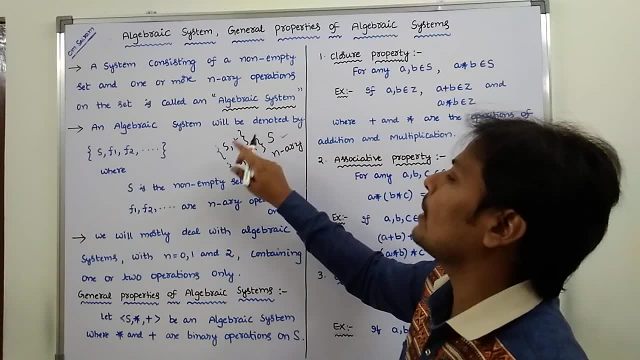 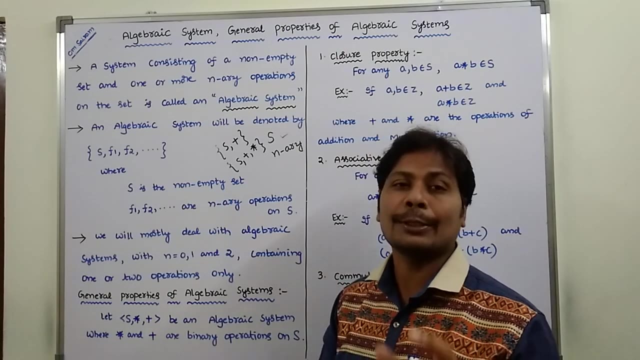 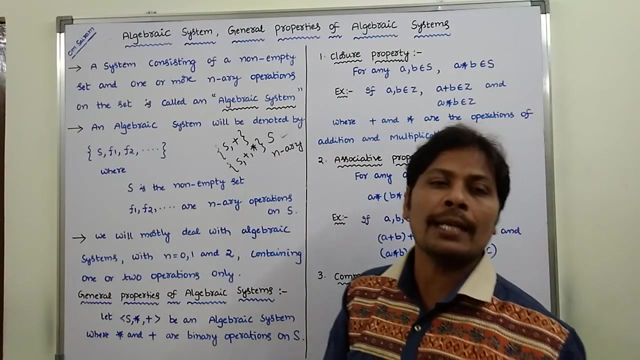 Here n is equal to 1 operation. The algebraic system which deal with only one addition operation performed on the set. Yes. Second case: the algebraic system which deal with two operations: addition and multiplication. These are performed, these operations performed on the non-empty set. 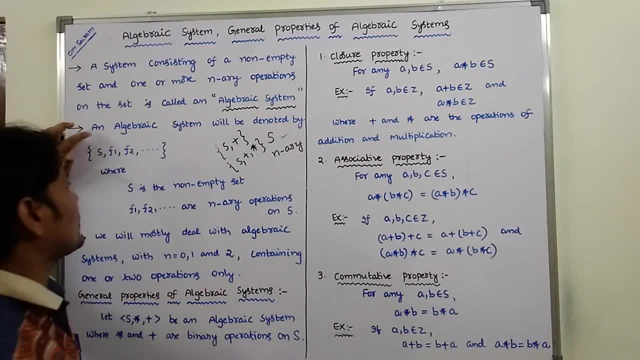 Yes, So generally algebraic system will be denoted by this one s comma, f1 comma, f2 comma, etc. Where s is the non-empty set: f1, f2, f3, etc. are n array operations on the set. Yes, We will mostly deal with. 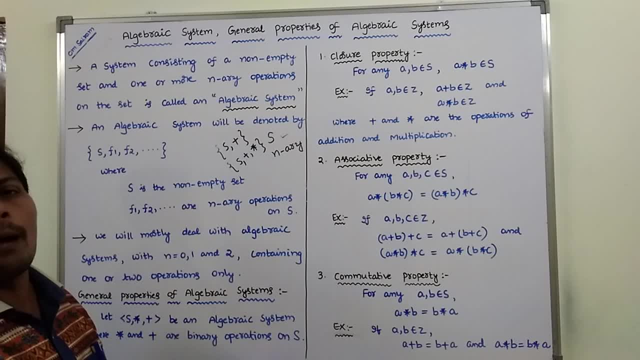 algebraic system with n is equal to 0 comma 1 and 2.. Here n is equal to 0 comma 1 comma 2.. Mostly algebraic systems which deal with no operation, with unary operation, with binary operation, n is equal to 0, is nothing, but only non-empty set is there. There is no operation. 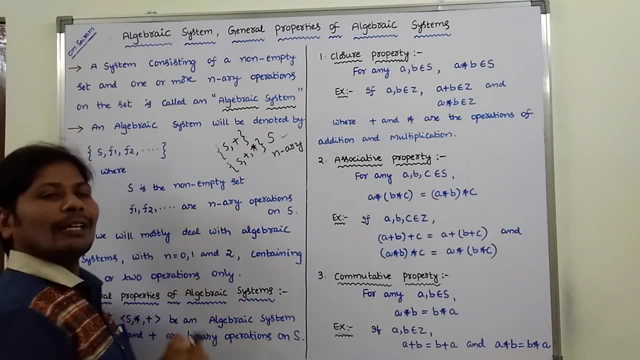 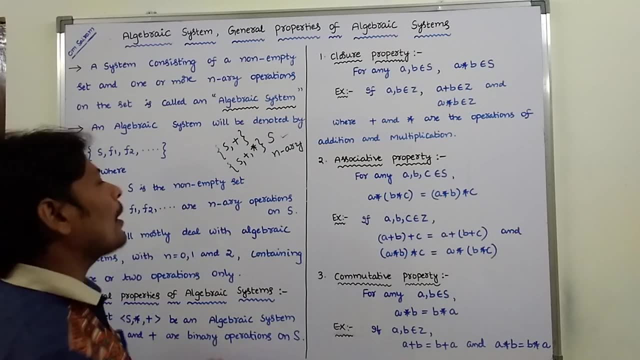 performed on the set Yes n is equal to 1 is nothing, but only one unary operation performed on the non-empty set Yes. илось Here also algebraic systems which deal with only non-empty set. in the set Here n is equal to 1.. 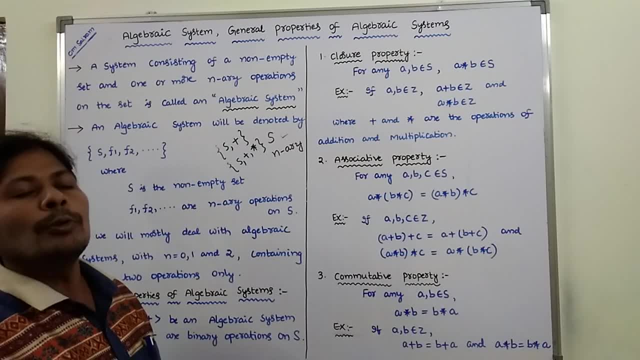 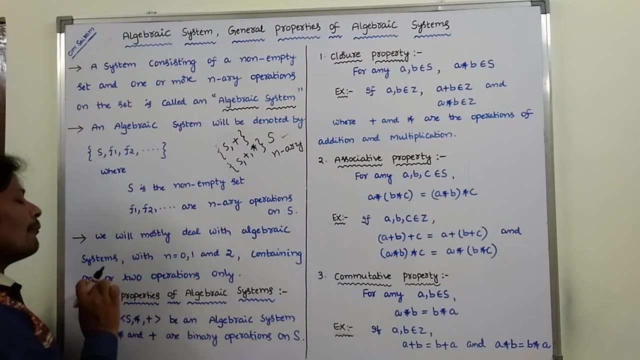 eii��니 and pearlsZizë for an image"or something else. question's similar to absolute, super strict. answer to two is nothing but two operations that can be performed on the non empty set. so this is the meaning of n array operation, but most of the algebraic systems deals with only one or two. 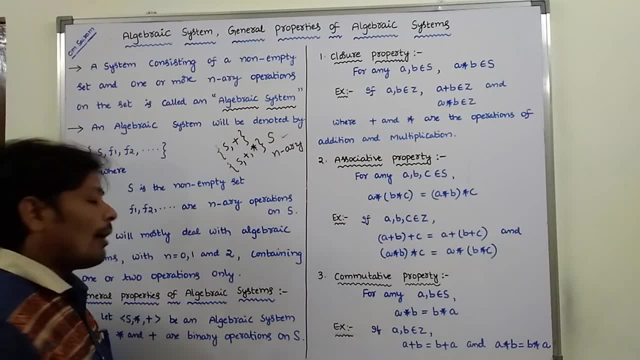 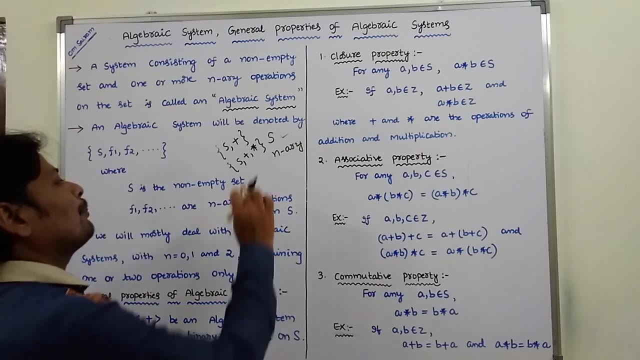 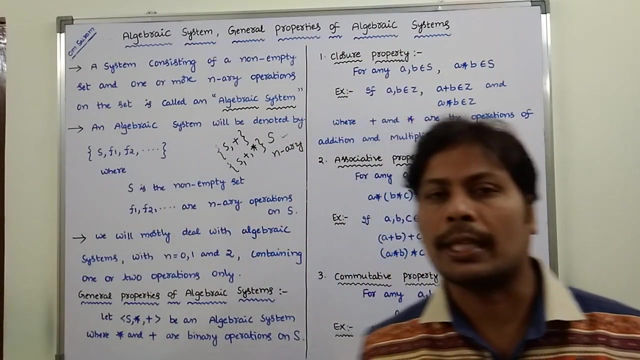 operations only. next, what are the general properties of the algebraic system? suppose we can take the algebraic system s comma plus, comma star, where s is the non-empty set, and plus and multiple plus and star are the binary operations that can be performed under non-empty set. yes, first, property, closure property. so closure property means we can take. 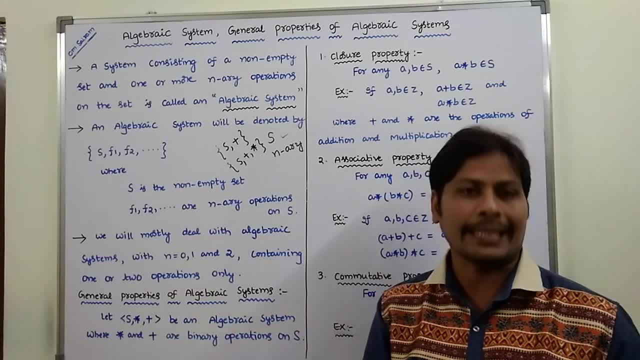 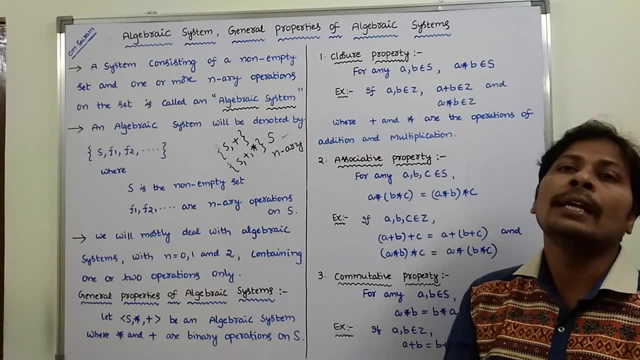 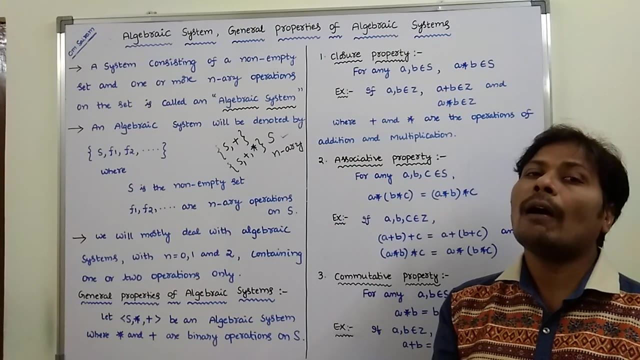 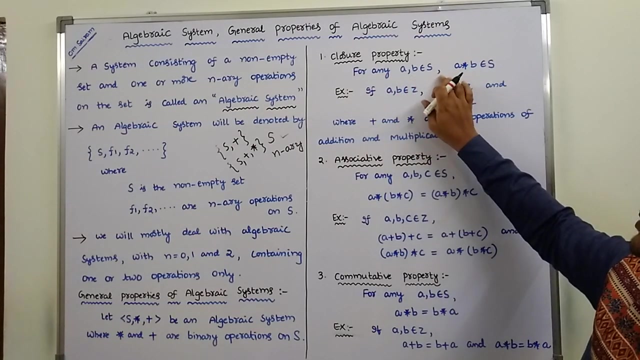 any two elements from the norm empty set: yes, so that is a and b. so a comma b belongs to s, then a plus b also belongs to s and a star b also belongs to. yes, closure property for any. a comma b belongs to s, a star b also belongs. 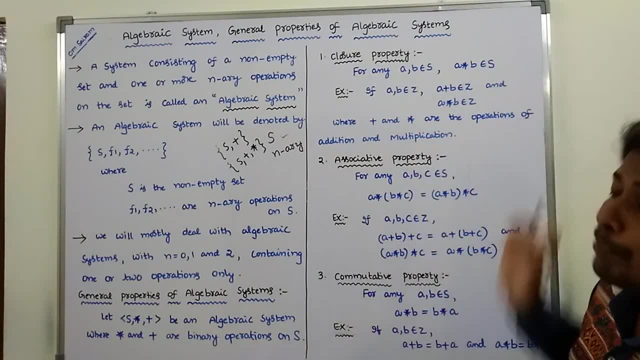 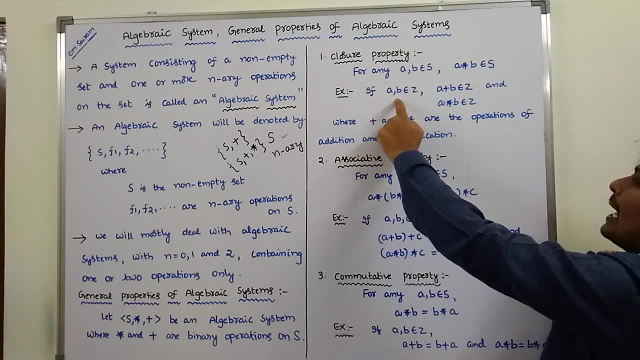 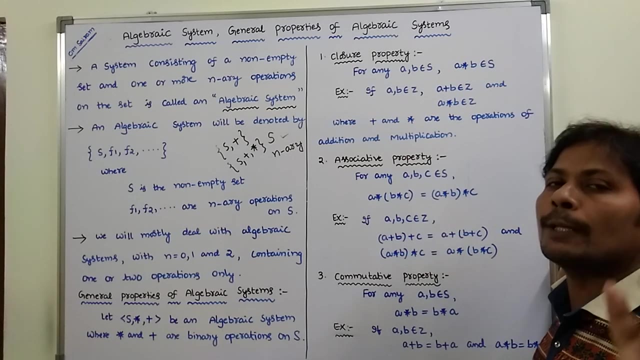 to yes, like a plus b also belongs to yes. so where, for example, is a comma, b belongs to z. z is nothing but set of integers. it contains both the positive elements and negative elements. so here a plus b belongs to z and a star b belongs to z. so this is the 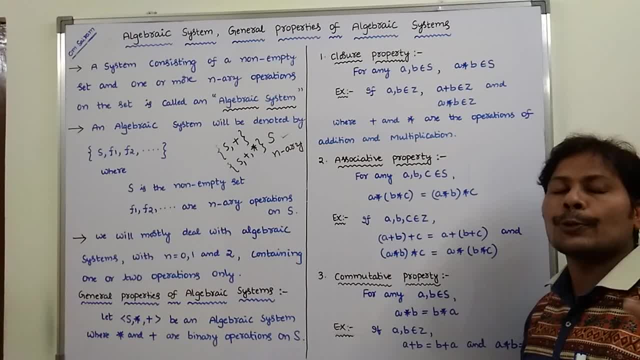 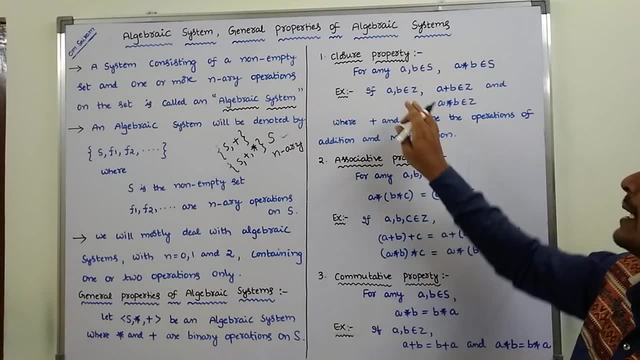 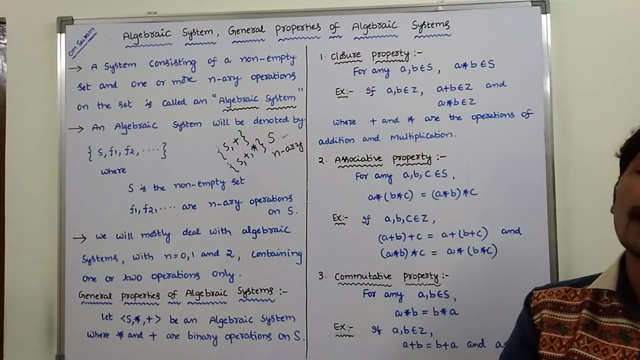 closure property. we can take any two elements from the set z, so that are a and b, so it can be written as a comma b belongs to z, then a plus b also belongs to z. a star b also belongs to z. okay, where plus and star are the binary operations of addition and multiplication. 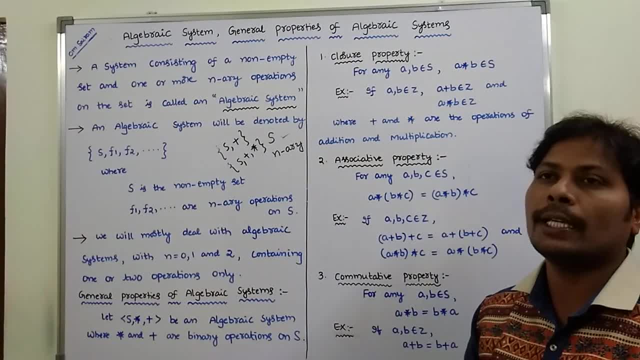 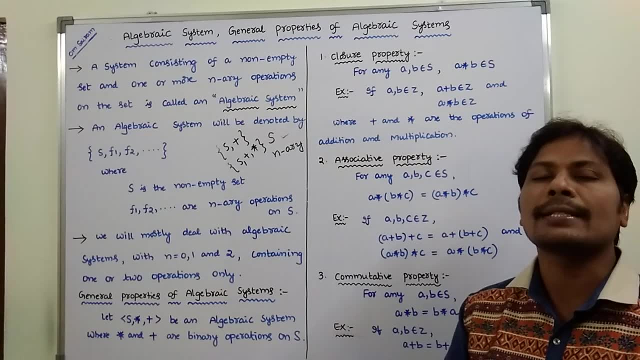 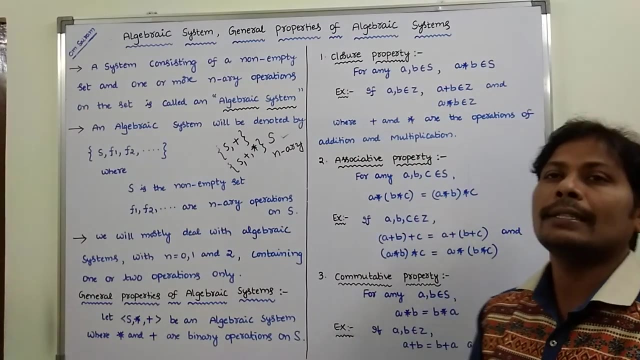 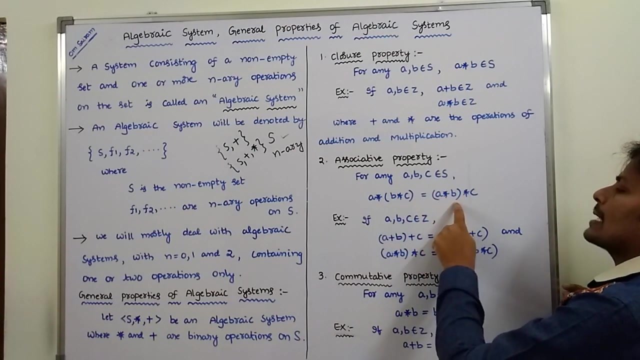 next second property, associative property, we can take any three elements- a comma b, comma c- from the non-empty set. yes, it can be represented as a comma b, comma c belongs to. yes, then it satisfies this proper condition. a star b, star c is equal to a star b- star c whenever this condition is satisfied. 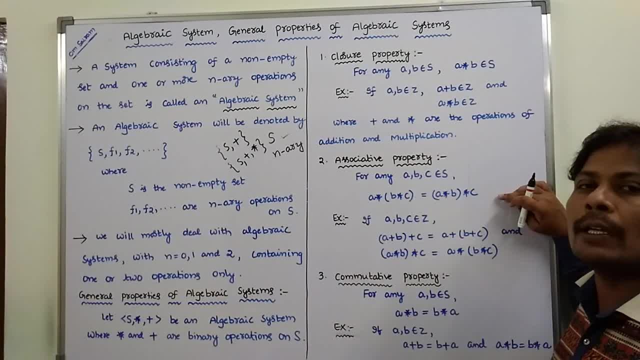 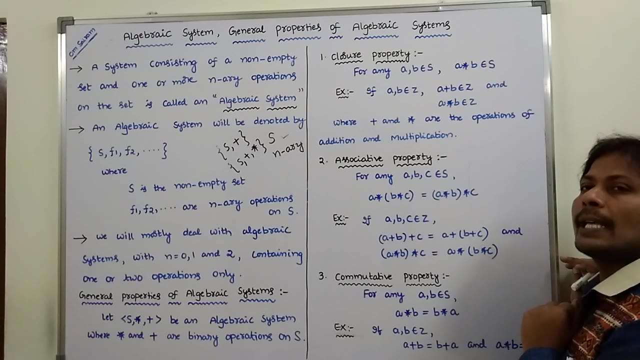 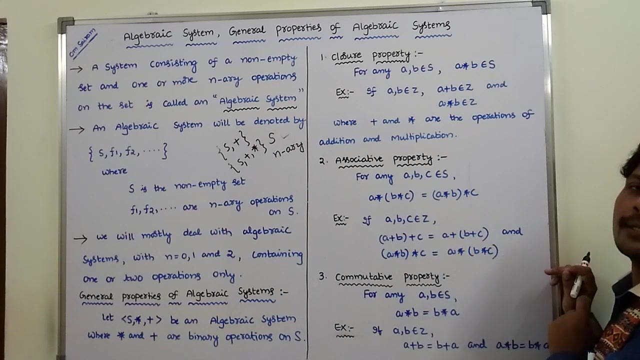 by the three elements that are taken from the non-empty set. yes, then plus and star operation satisfies the associative property. for example, we can take three elements from the set of integers z. then we have to check the addition operation is associative and the multiplication operation is associative by satisfying this condition. so a plus b plus c is equal to a plus b plus c whenever. 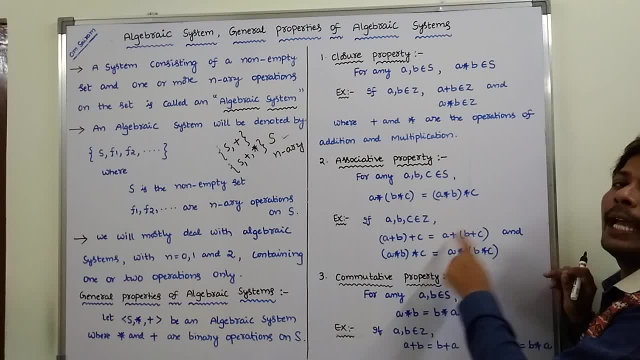 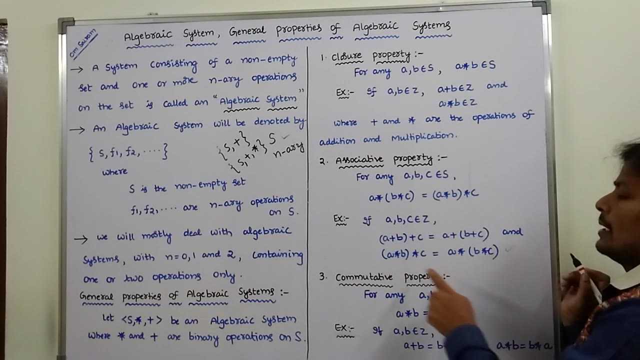 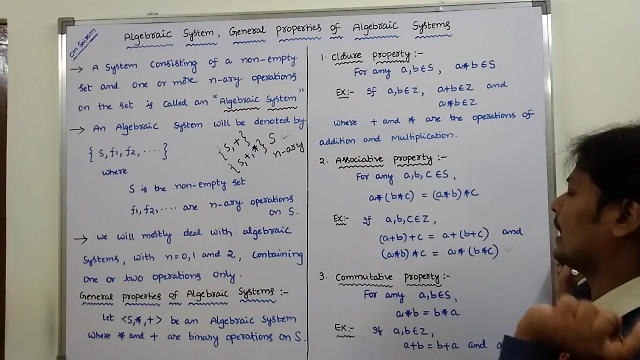 this condition is satisfied, we can say that addition operation is associative. next, a star b star c is equal to a star b star c, whenever this condition is satisfied, is associative. on the set: yes, okay, on the set: general, okay. third property is commutative property. we can take any two elements from the non empty set: yes, it. 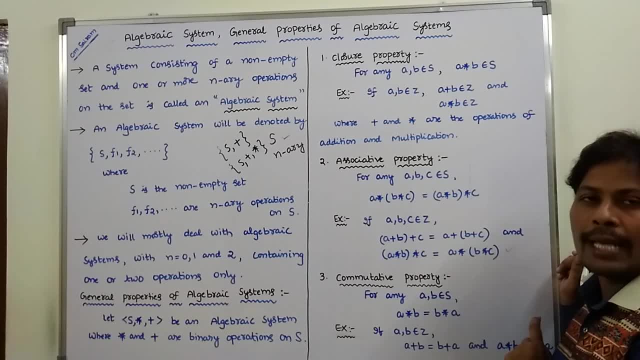 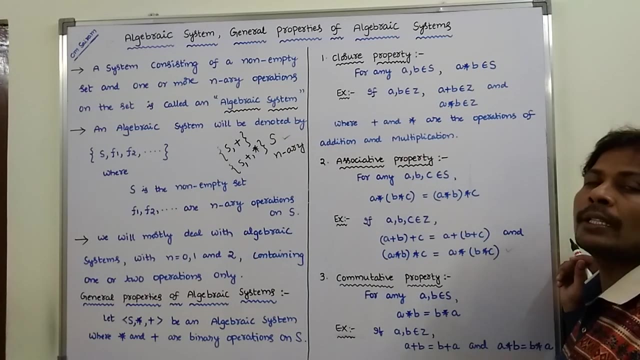 can be represented as a comma. B belongs to yes. then it satisfies the following condition: yes, army is equal to B star ye. whenever this condition is a satisfied, the multiplication operation is commutative. okay example: we can take any two elements from the norm empty set jet. so that is a comma. B belongs to jet. 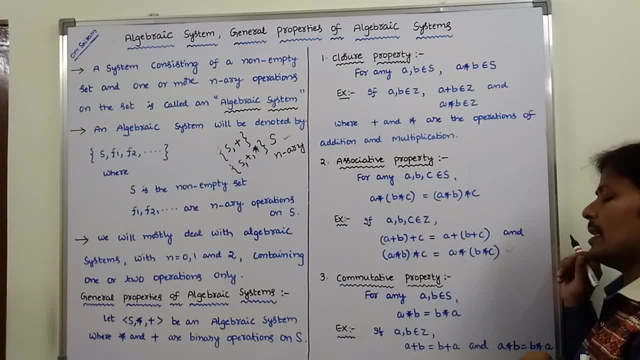 then it satisfies the following condition. so a plus B is equal to B plus a. so if the condition is satisfied, the addition operation plus is commutative on the non empty set general and a star B is equal to B star gay. here, if the condition is satisfied, the multiplication operation is a. 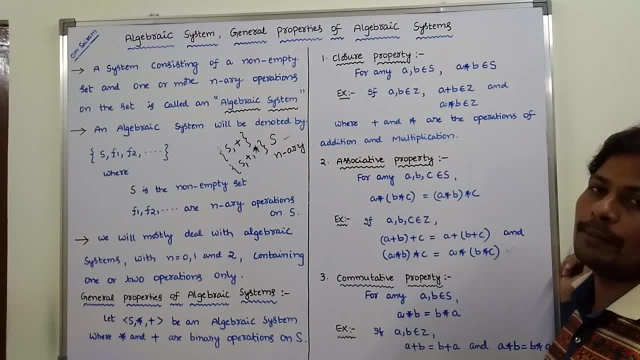 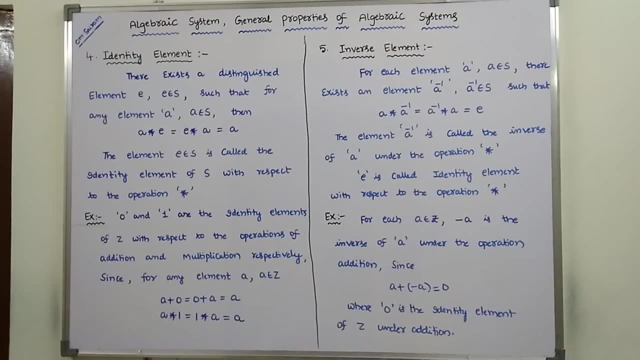 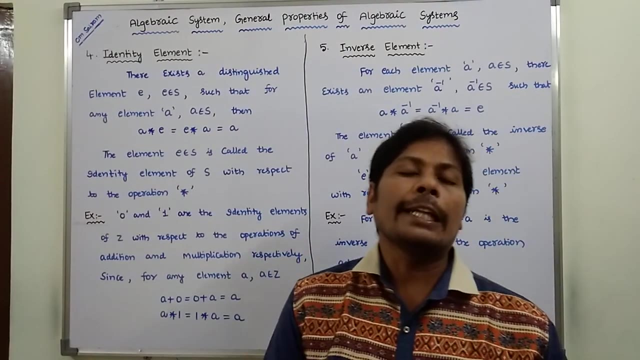 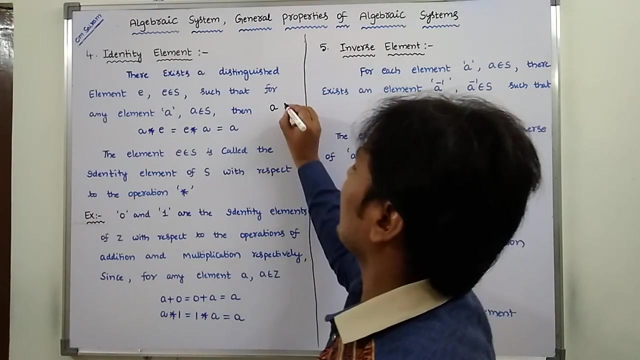 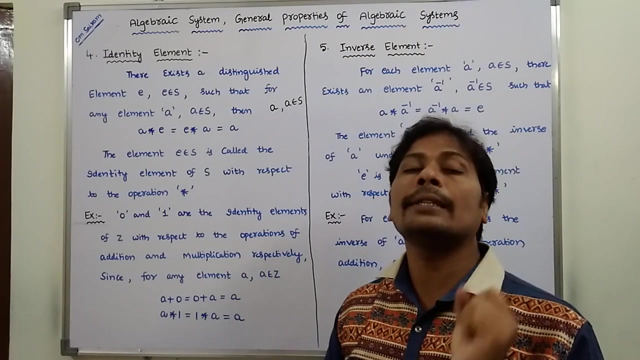 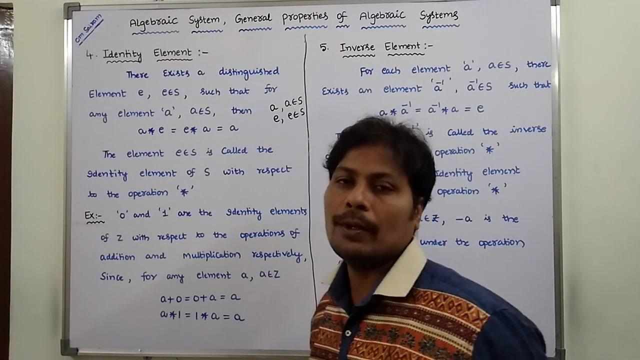 commutative under the set general. okay. next property is identity element property. suppose we can take an element a, so that is a belongs to yes, and also we can take and distinguish the element that is a E, E belongs to S. Okay, Then A star, E is. 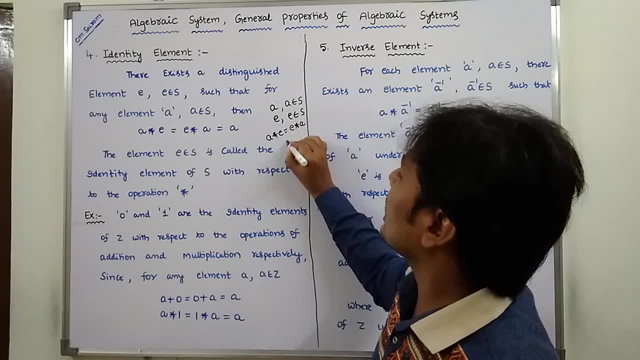 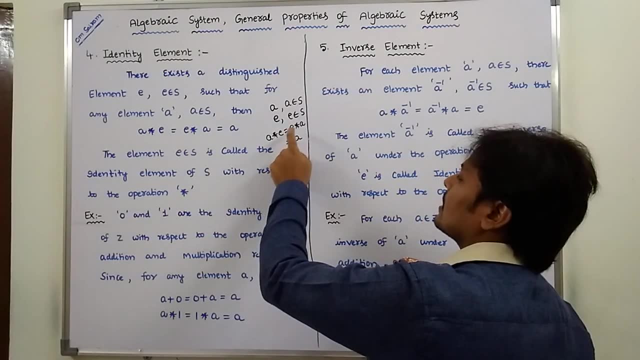 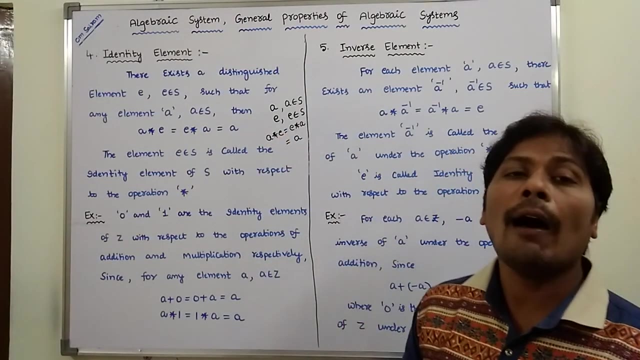 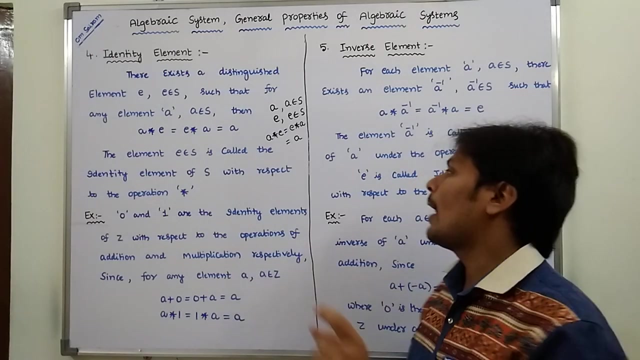 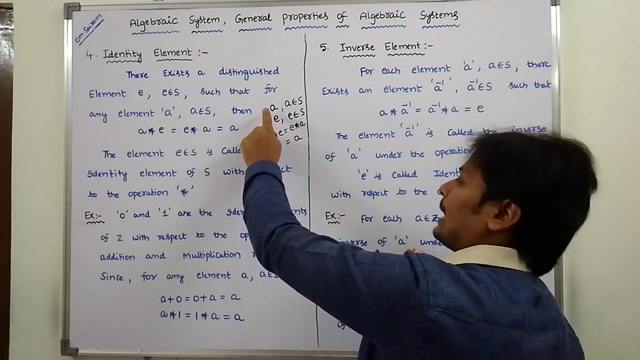 equal to E. star A is equal to A, So then it satisfies this condition. So A star E is equal to E, star A is equal to A. where E is called the identity element, That identity element also belongs to S under the operation star. Okay, So let us take an element A. 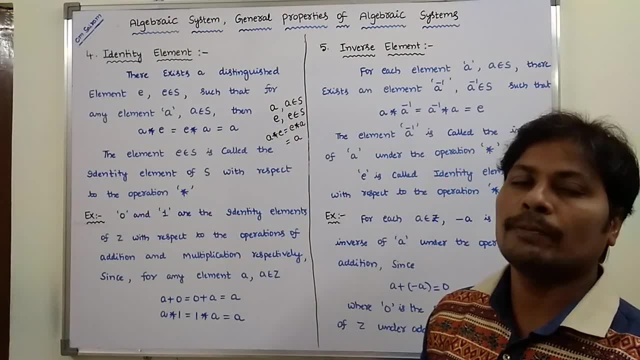 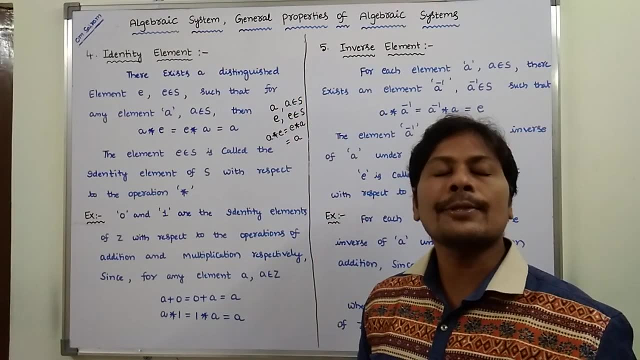 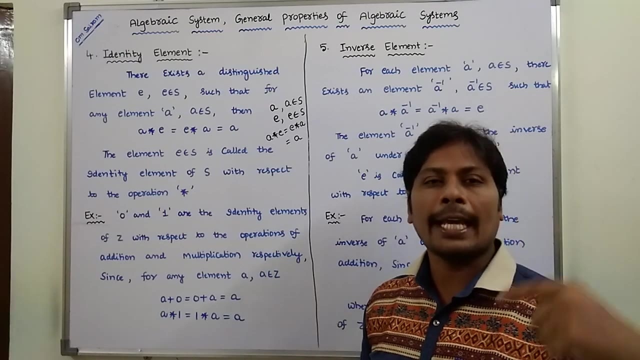 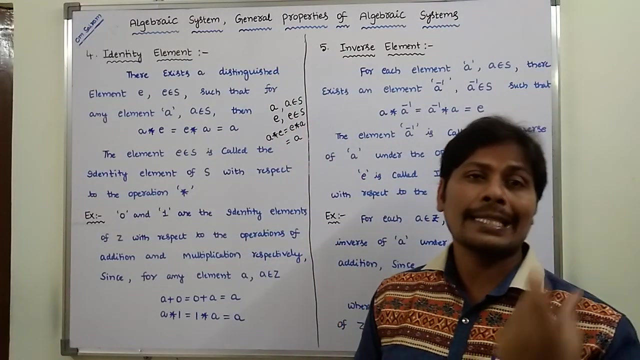 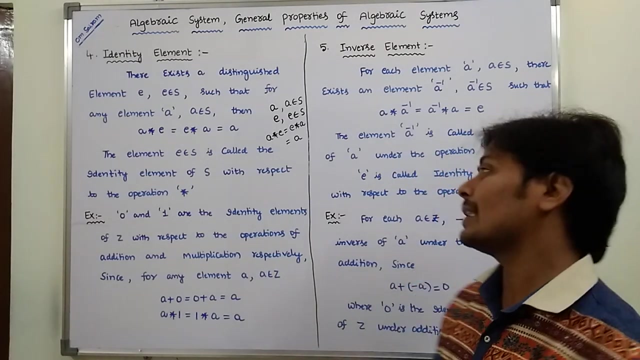 A belongs to S. That means element A is taken from the non empty set, yes. and also we can take an distinguished element, that is E. E is also taken from the non empty set, yes. therefore E belongs to yes. then it must satisfy the condition. A star E is equal to E. star A is equal to A, here E. 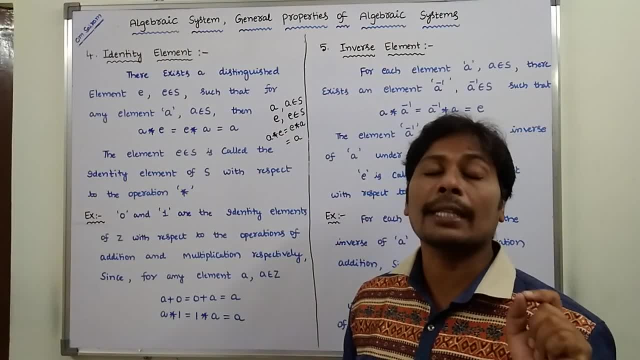 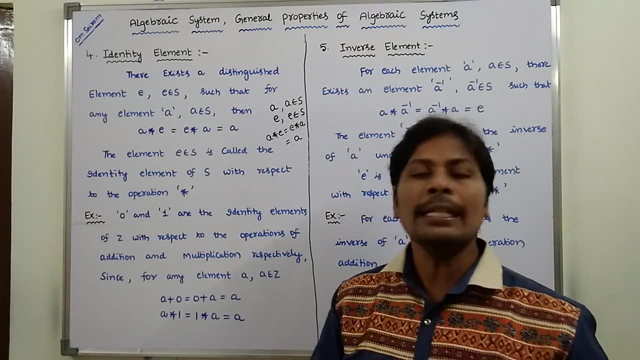 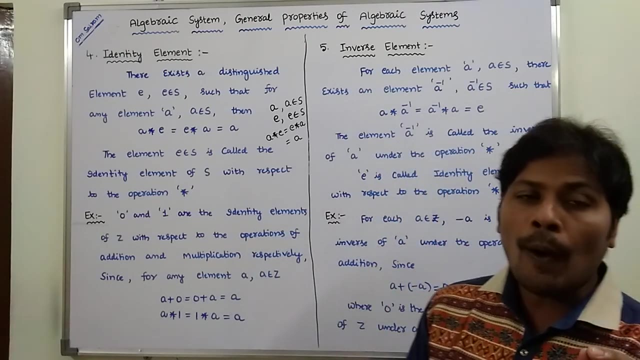 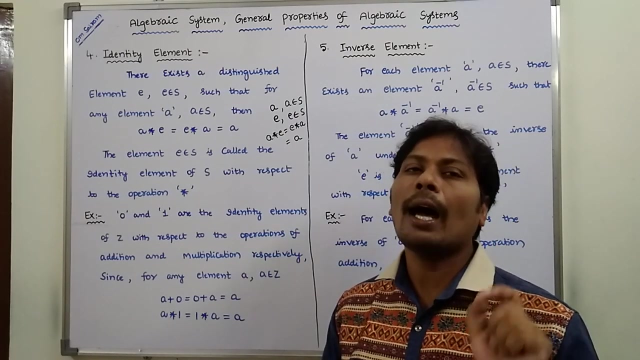 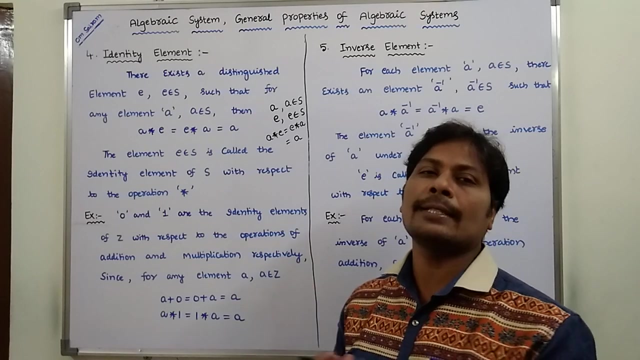 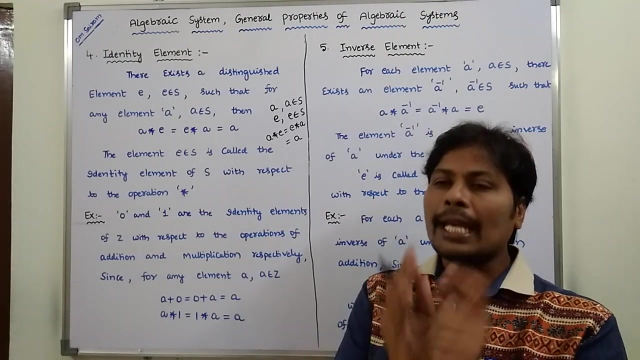 is called the identity element with respect to the operation multiplication. okay, so this is the identity element property. okay, next example. so here 0 & 1 are the identity elements with respect to the addition operation and multiplication operation. so for addition operation, the identity element is 0. for multiplication operation, the identity element is 1, so these: 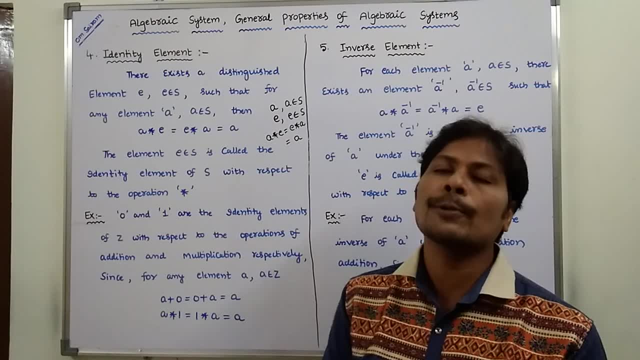 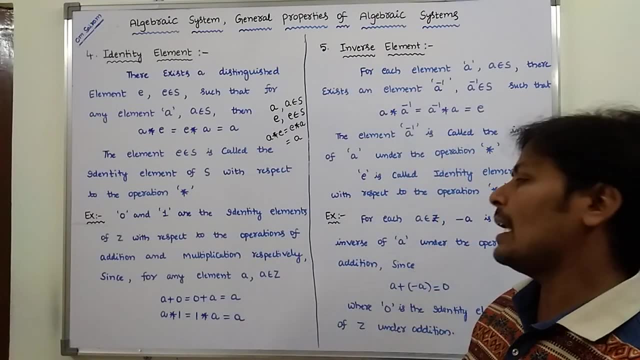 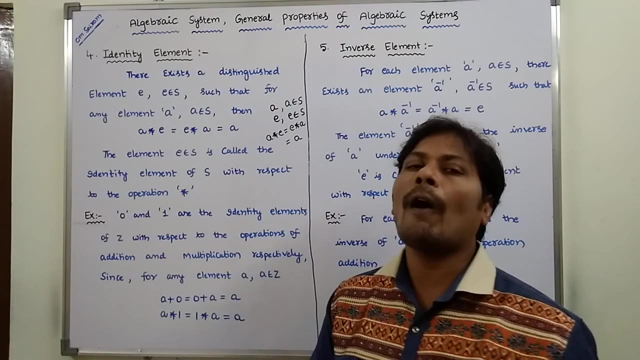 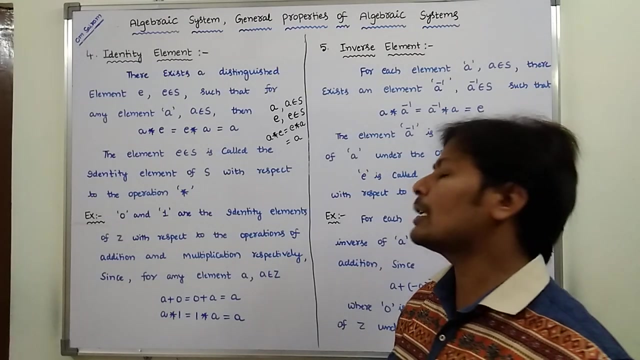 identity elements 0 and 1 also belongs to z with respect to the operation addition and multiplication, then it must be set, for we can take any element a that is taken from the non-empty set z, so that we can take a belongs to z. okay, it must satisfy these two conditions. a plus 0 is equal to. 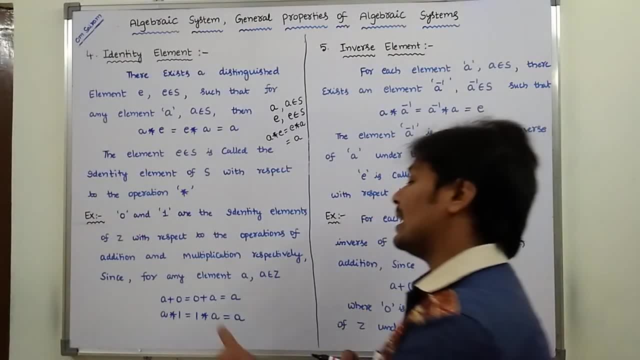 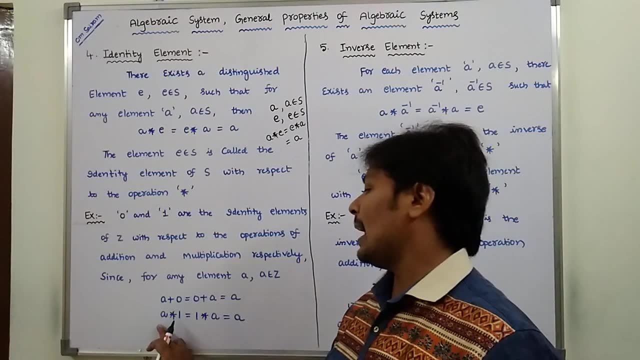 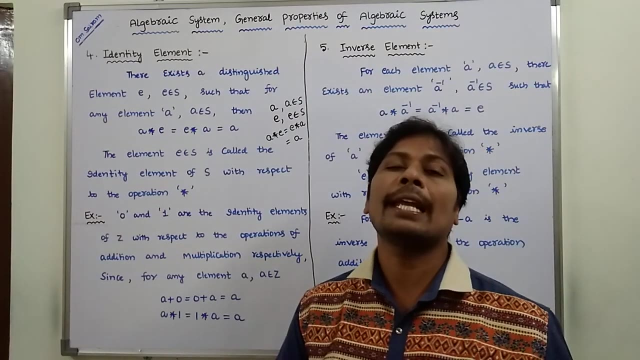 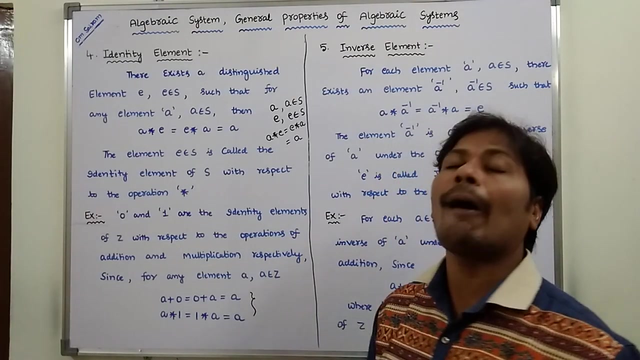 0 plus a is equal to a, here 0 is the identity element with respect to the addition operation. next, a star 1 is equal to 1. star a is equal to a, here 1 is the identity element with respect to the multiplication operation. so whenever these two conditions are, 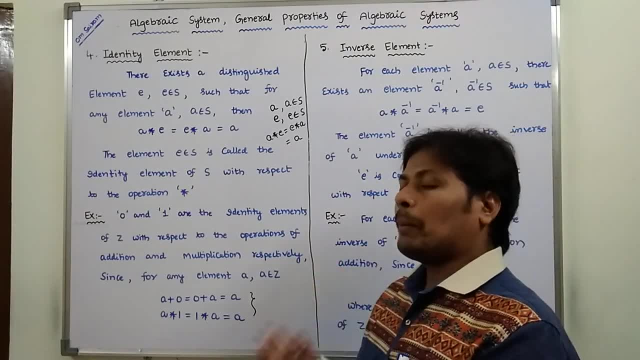 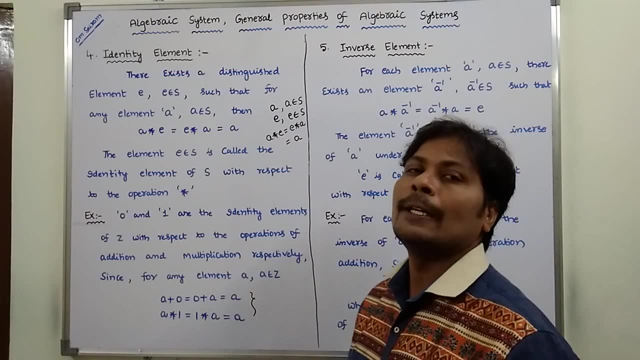 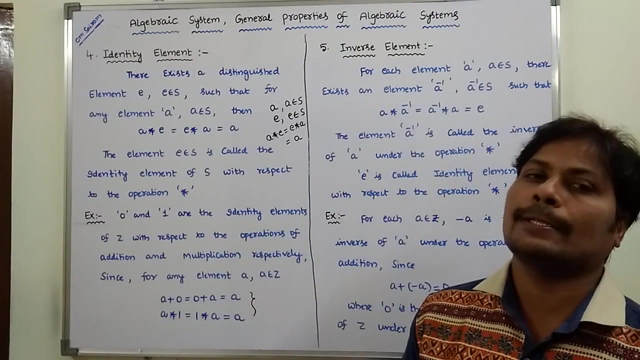 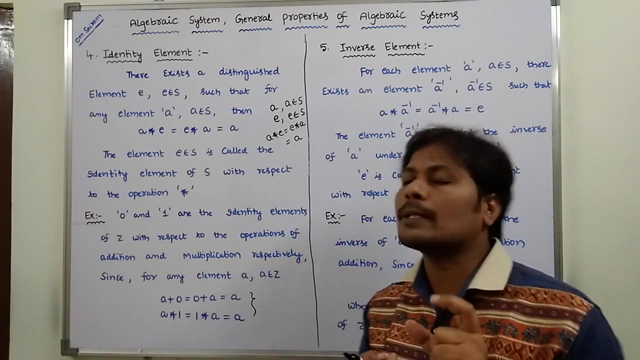 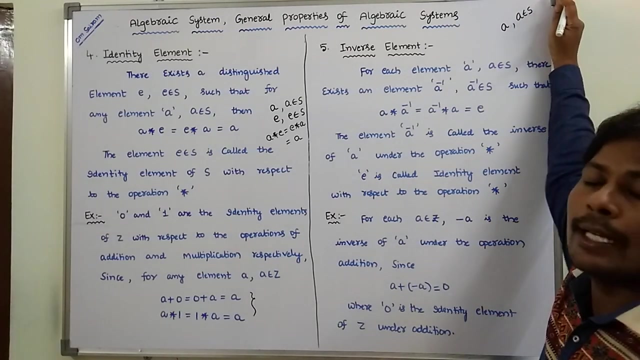 satisfied then. so plus operation and multiplication operation satisfies the identity element property under the set general jet is nothing but set of integers. next first property is inverse property. okay, so suppose we can take an element gain so it belongs to. yes, that means element, the air is taken from the 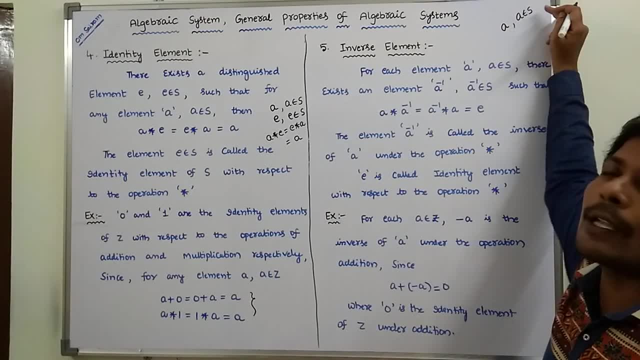 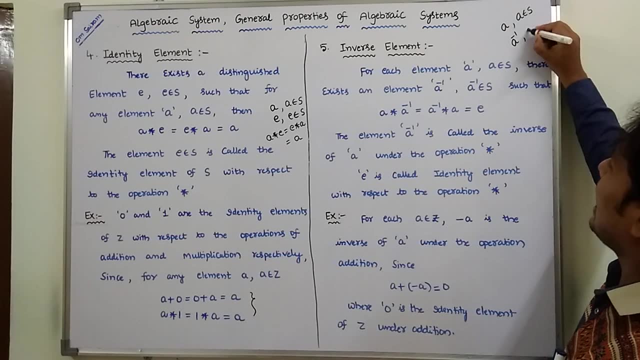 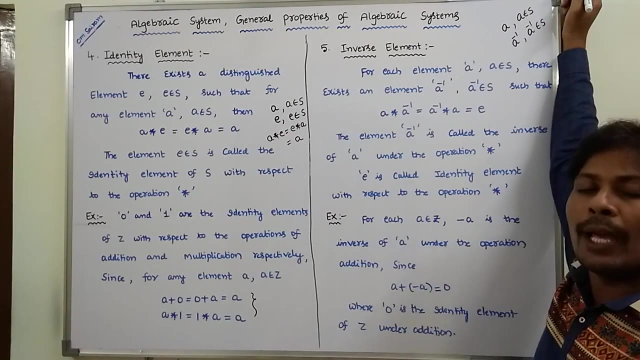 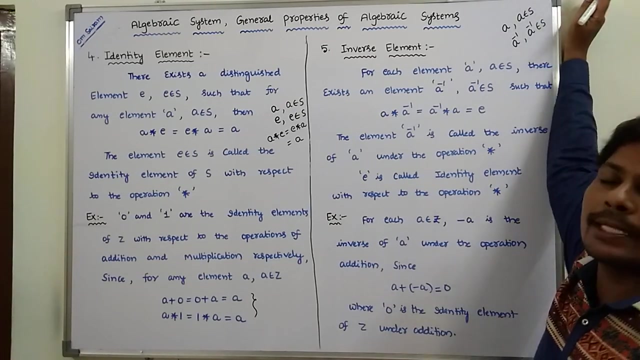 set yes, so the days he belongs to yes. next, we can take another element that is a inverse. a inverse is a a belongs to yes. okay, that means we can take two elements from the norm empty set. yes, one is the a element, so a belongs to yes. we can take another. 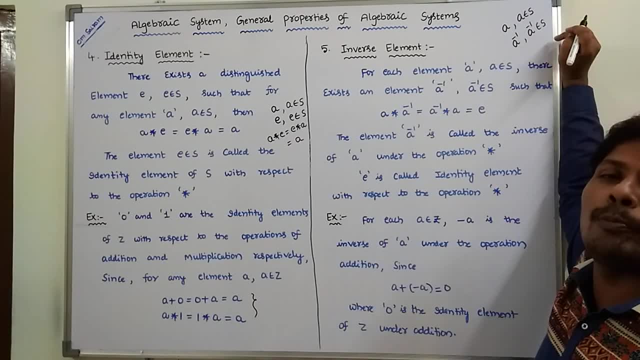 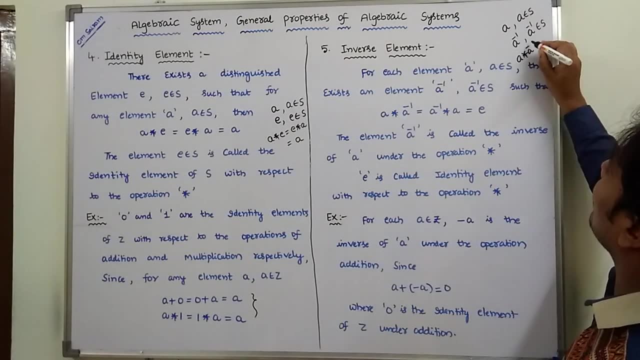 element a inverse. a inverse also belongs to yes, then it must satisfy the condition. a into a inverse is equal to a. inverse into a is equal to e. so this is the e is called the identity element. with respect to the multiplication operation. a into a plus is equal to a inverse into a is equal to e. e is: 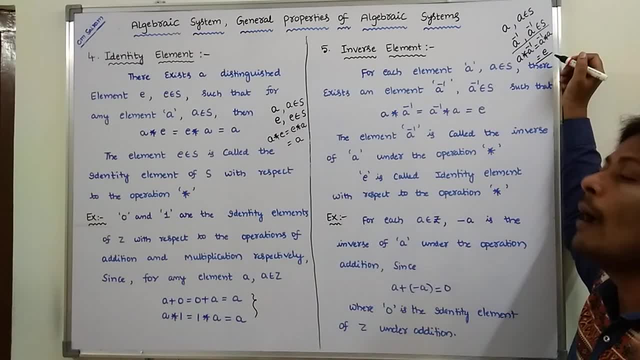 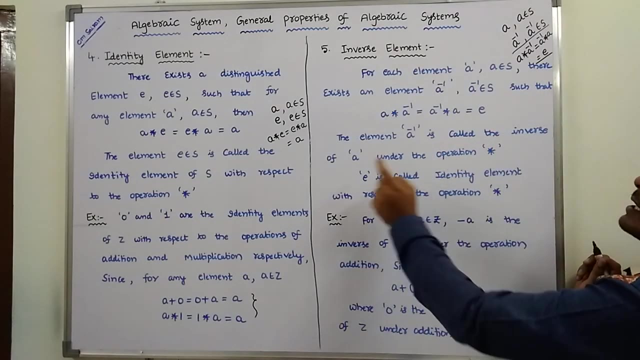 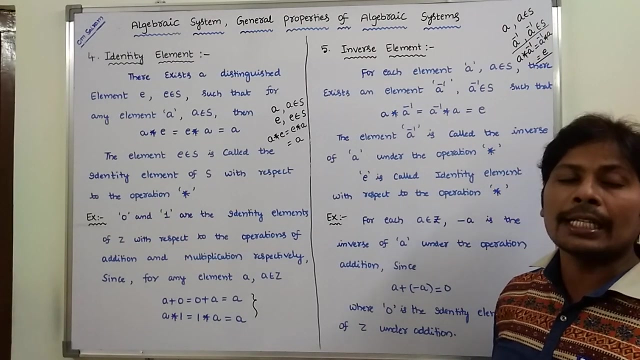 nothing but identity element with respect to the multiplication operation, where a inverse is called the inverse. inverse of a. okay, inverse of revelier, okay, a inverse, all the inverse of cables, a under the operation when application ie called the identity element with respect to the multiplication operation. so e is equal. 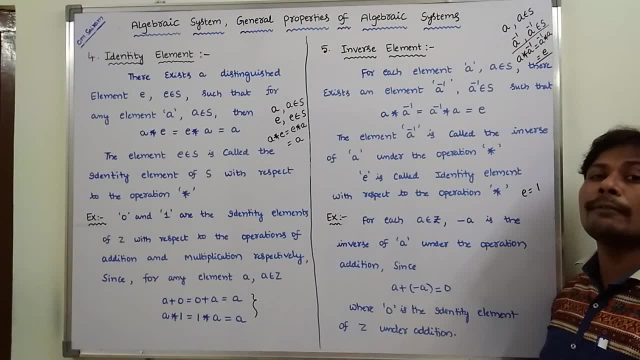 to 1, because identity element 했던 perspective to the multiplication operation is 1.. Okay, Example: suppose we can take two elements from the non-empty set Z. So one element is A, A belongs to Z, and another element is: 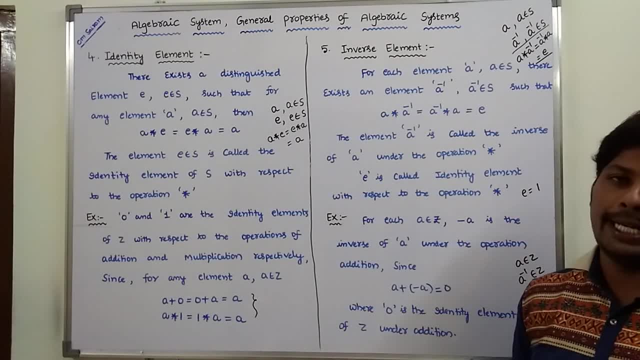 A inverse. A inverse belongs to Z. Okay, Then A plus minus A is equal to E. Okay, So minus A is the inverse of element A. Okay, Here E is nothing but identity element with respect to the operation plus, So we can write it as: A plus minus A is equal to 0. 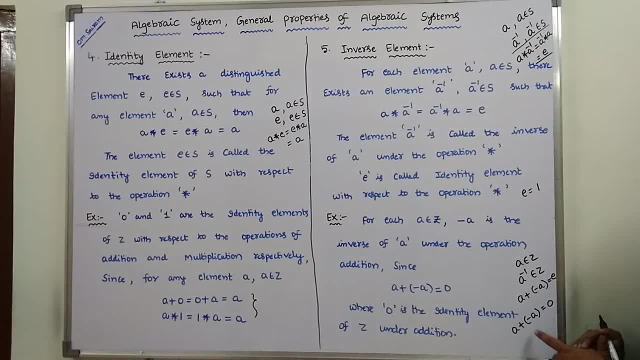 Okay, So A plus minus A is equal to 0.. Minus A is the inverse of A under the operation Z. Okay, So therefore A plus minus A is equal to E. That means A plus minus A is equal to 0.. 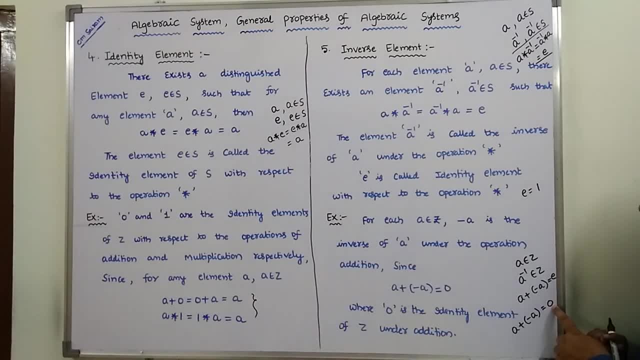 Here, 0 is nothing but identity element with respect to the operation plus. Okay, So this is the inverse element property. Same way. so A into A inverse is equal to E. Okay, So when E is the identity element with respect to the operation multiplication, So that 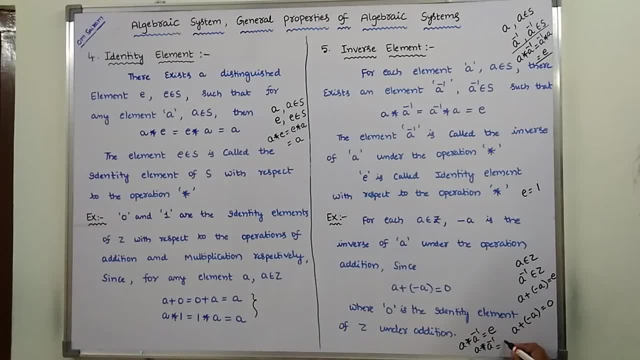 is A into A inverse is equal to 1.. Because here E is nothing but identity element. with respect to the multiplication operation, that value is 1.. So that A into A inverse is equal to 1.. Okay, So this is the inverse property. inverse element. So this is the inverse property. 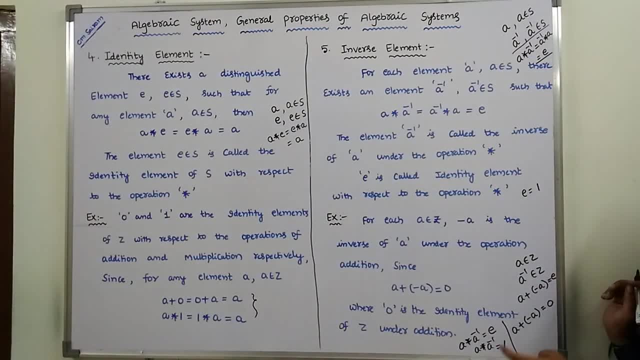 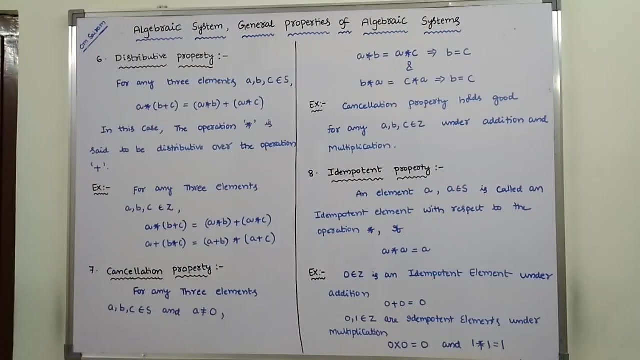 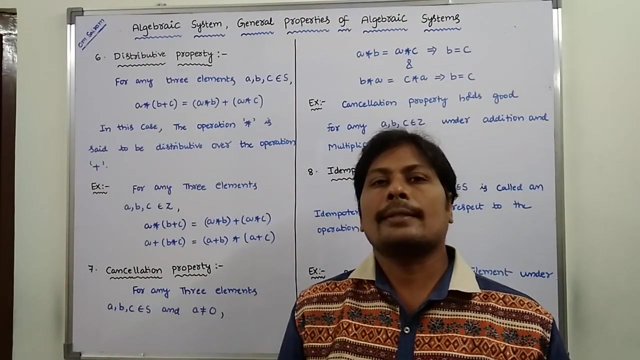 property. Whenever these two conditions are satisfied, then we can say that element a has the inverse minus a, Element a has the inverse minus a. These two elements, a and a inverse, also belongs to z. Okay, Next property is distributive property, So we can take any three elements. So 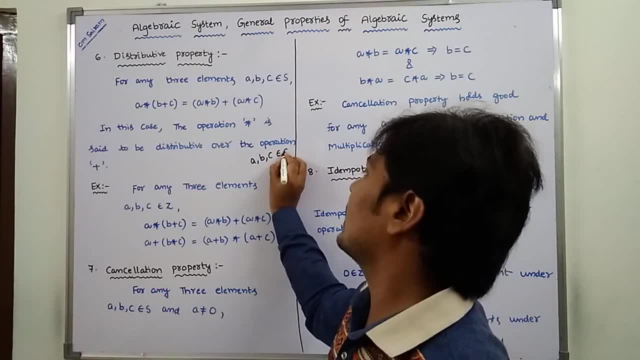 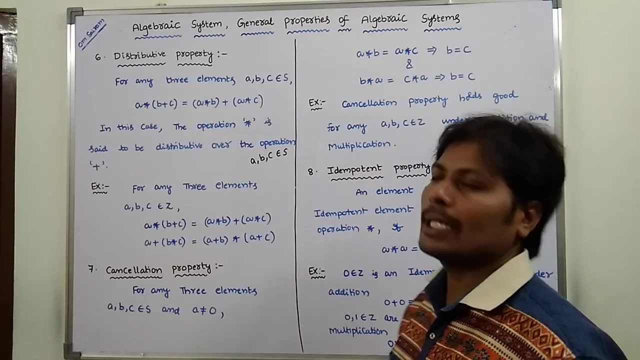 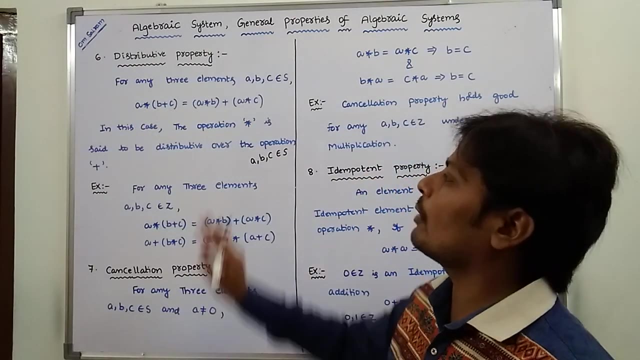 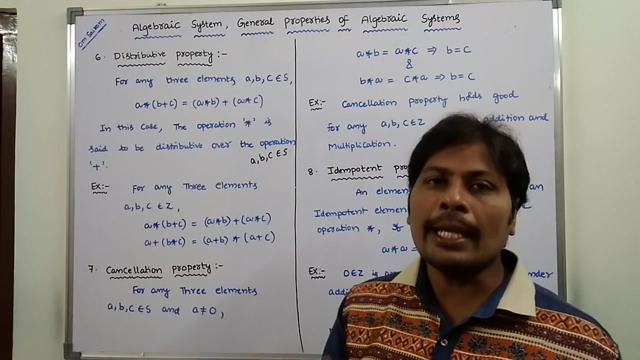 a b c from the set non-empty set. yes, that is represented as a b, c belongs to yes, Then the distributive property is a star b plus c is equal to a star b plus a star c. So for any three elements that are taken from the non-empty set, a comma b, comma c. 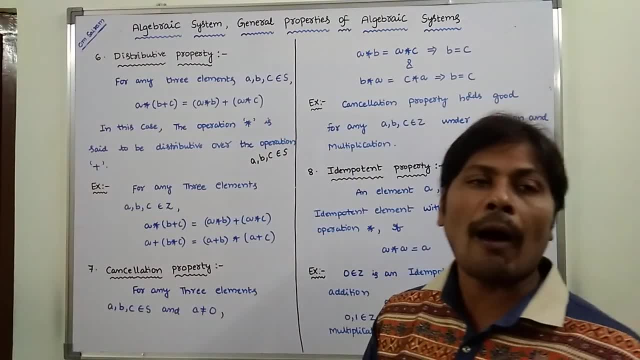 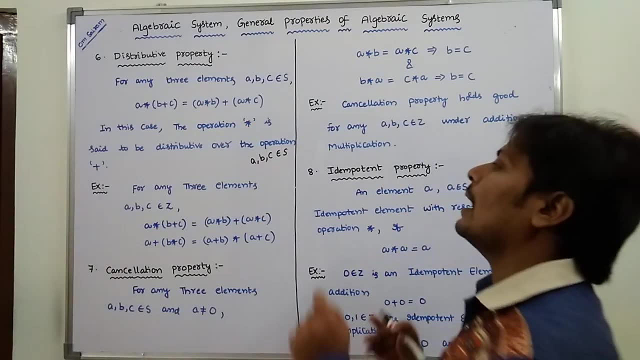 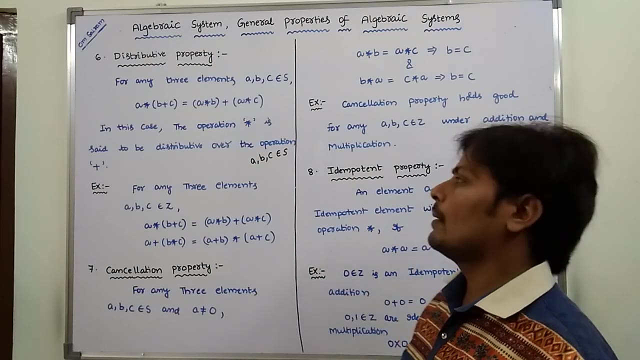 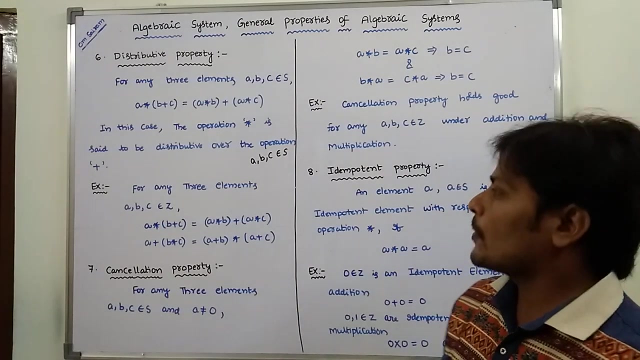 it satisfies this condition. a star b plus c is equal to a star b plus c. Here the operation star is a distributive over plus Okay. The operation star is a distributive over the operation plus Okay. So example for any three elements, a, comma, b, comma c belongs to. 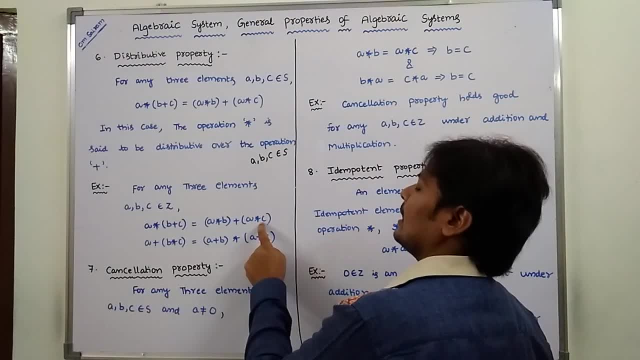 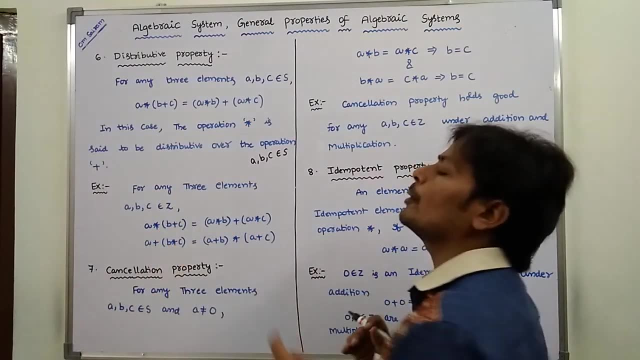 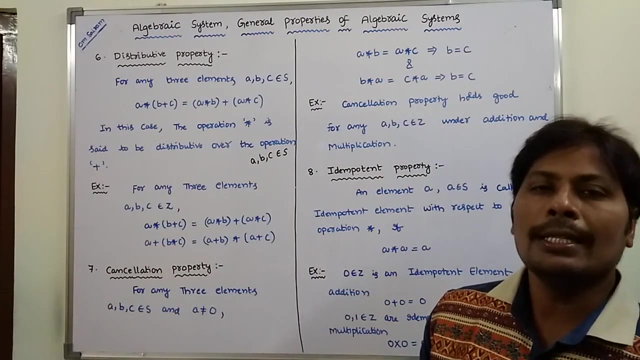 z. So it satisfies this condition and this condition Here. this condition is: a b, c belongs to z. So a b, c belongs to z. Okay, The operation star is a distributive over plus. The second case, the operation plus, is a distributive over star. So a star b plus c is. 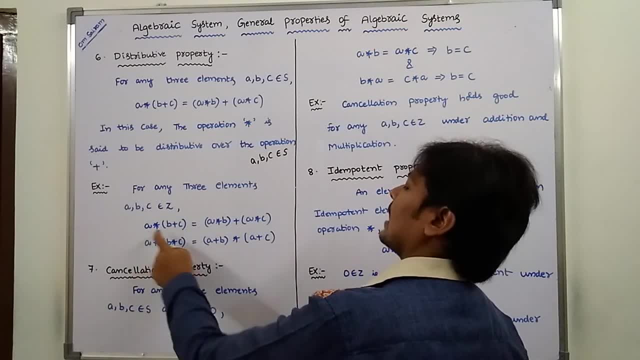 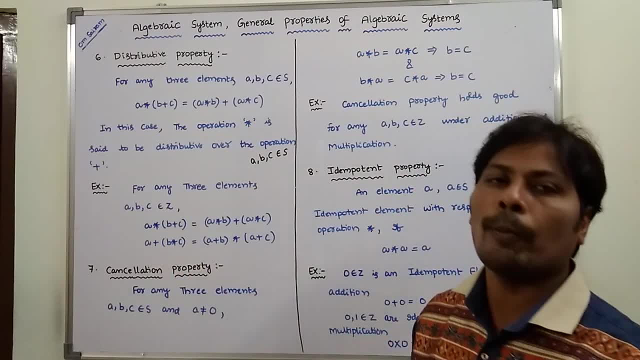 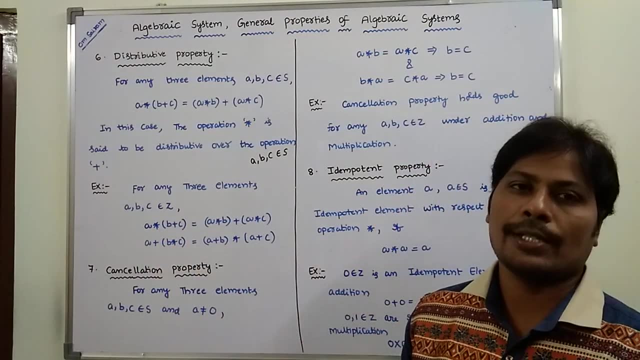 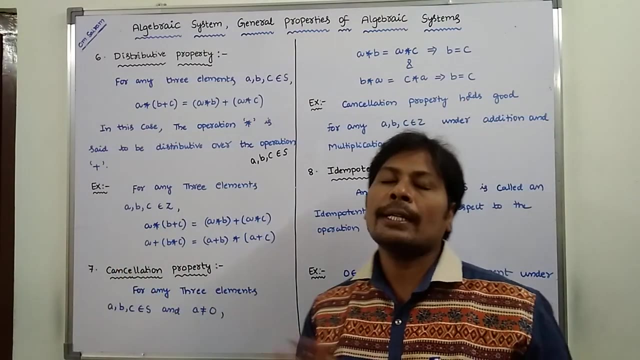 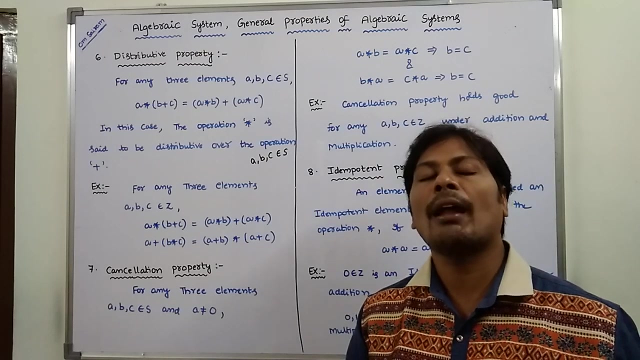 Okay, The operation plus is distributive over the operation star. Here. this is the operation star is distributive over the operation plus. Okay, So this is the distributive property. Okay, Next property is cancellation property For any three elements: a, comma, b, comma, c belongs to yes and a compulsory not equal to zero. 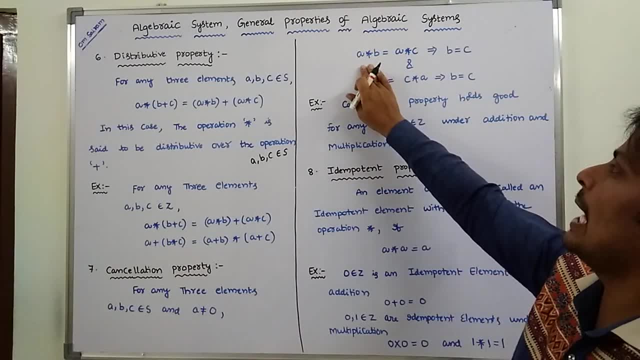 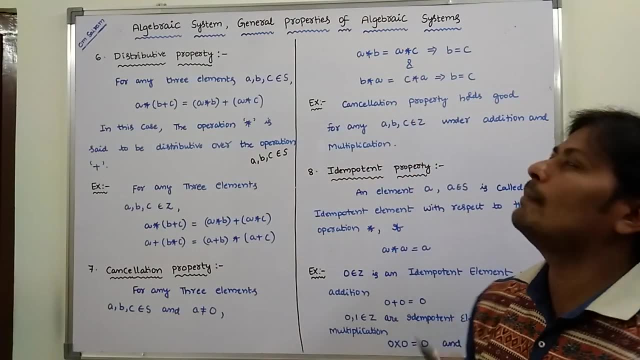 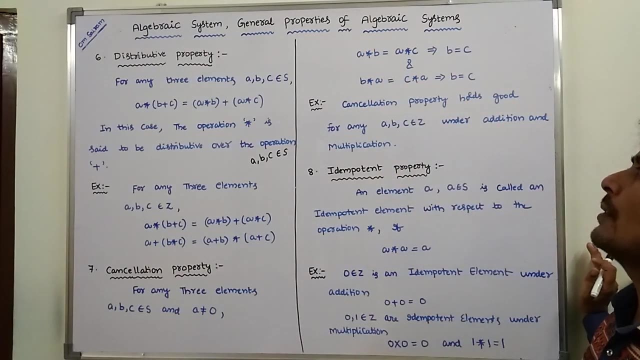 Okay, Then the cancellation property is a star b is equal to a star c. So left hand side and right hand side, same element a is there. We can cancel that element. The remaining elements are b equal to c. Okay, In the same way, b star a is equal to c star a. 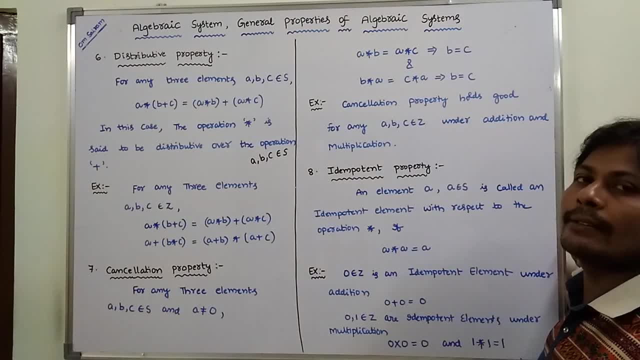 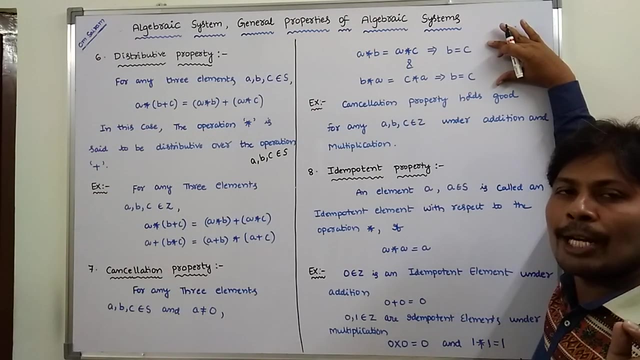 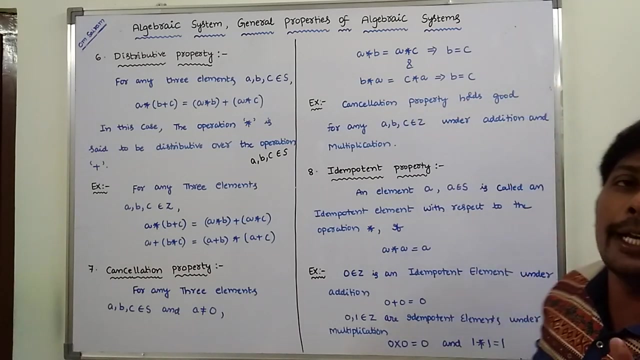 Left hand side and right hand side, same elements are there. That same elements are cancelled. After that We get that. we are getting. the result b is equal to c. Okay, So this is called as the cancellation property. So the cancellation property holds good for the set of integers z under the operation addition and multiplication. 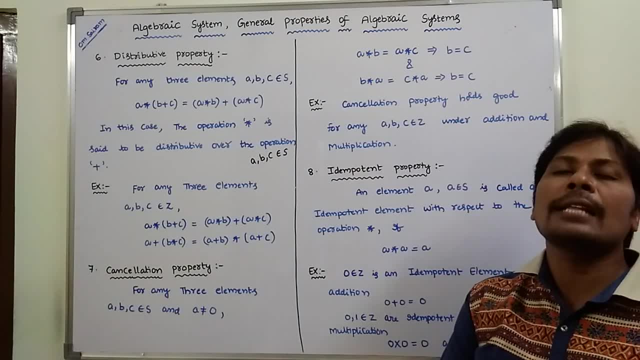 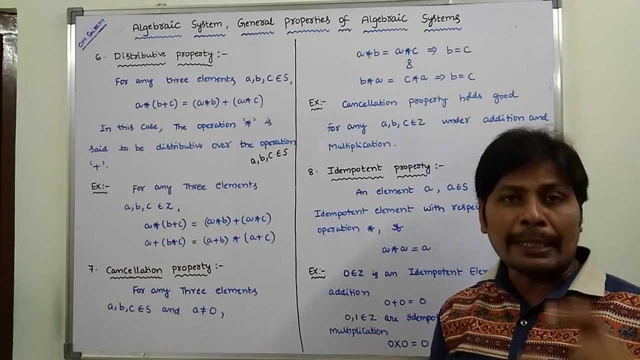 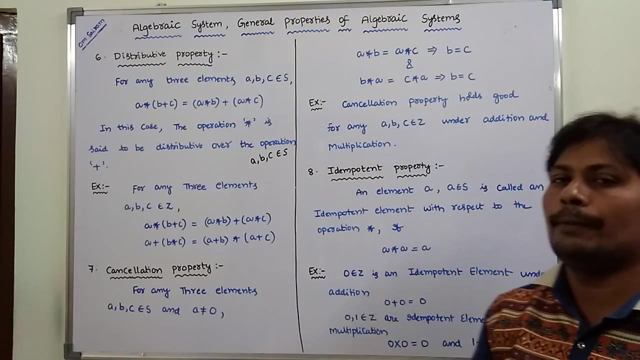 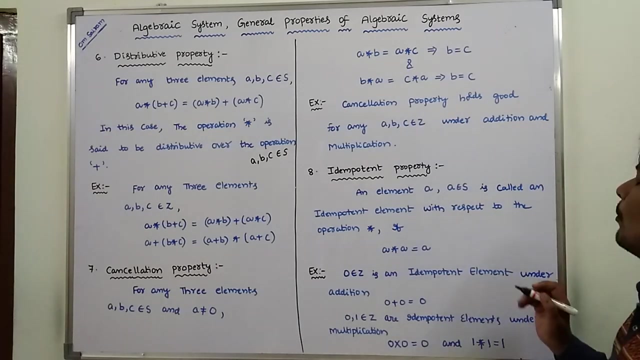 Okay, With respect to the addition operation, cancellation property is satisfied by this set of integers z. With respect To the multiplication operation, the cancellation property holds good for the set of integers general. Okay, Next, property is idempotent property. Okay, Suppose we can take an element a so from the non empty set. yes, 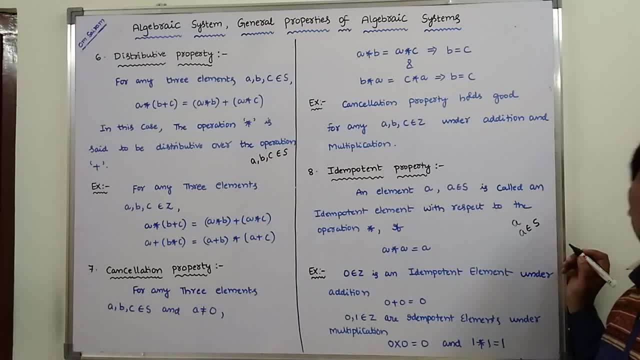 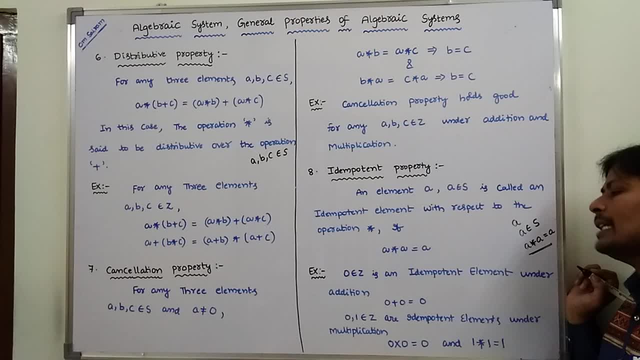 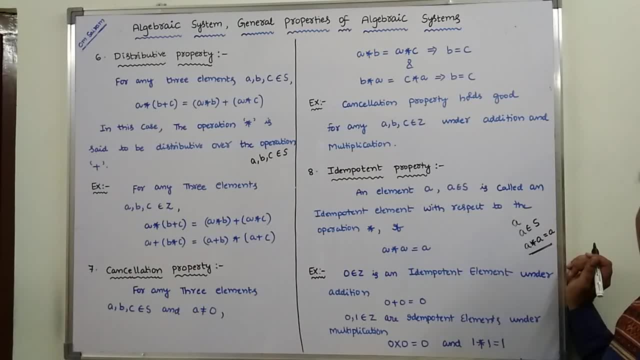 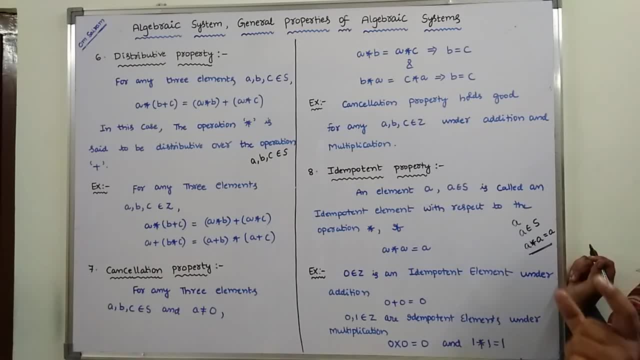 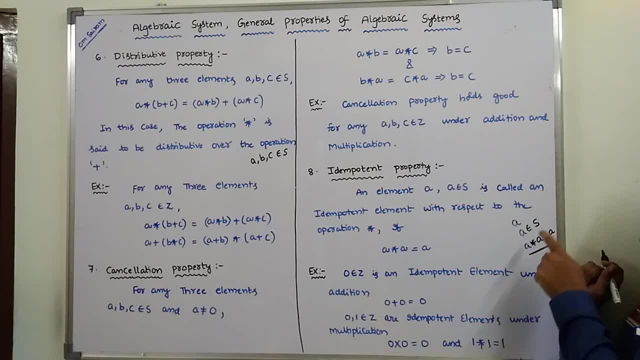 Then a star a is equal to a. Whatever the element you are taking, the same element is multiplied with the same element, Then we are getting the same element as the result. Okay, A star A is equal to A under the operation star. 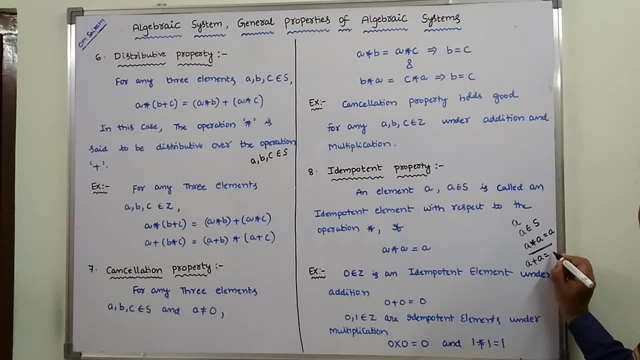 In the same way, A plus A is equal to A. Here the operation is addition operation. A plus A is equal to A. We can take an element A. The same element is added with the element A. We are getting the same result. 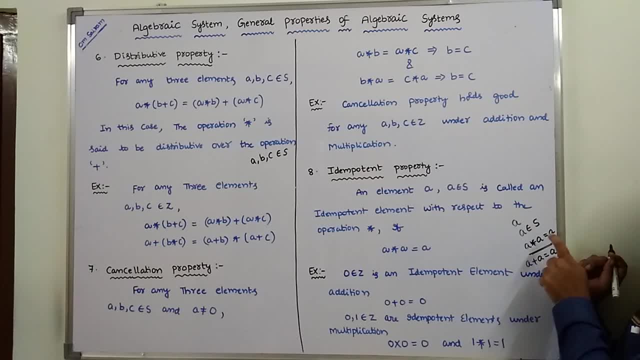 We are taking element is A. This element is multiplied with the same element, Then we are getting the result: also same element. So this star operation is idempotent, Okay, Next, Well, we can take an element A, So that element is added with the same element. 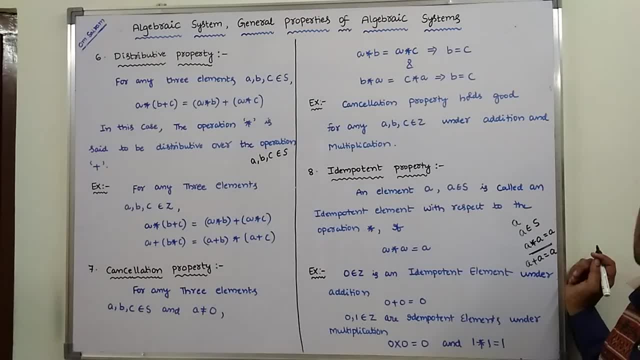 Then we are getting the result. also the same element. Then it is called as idempotent property. Okay, For example, 0 belongs to Z is an idempotent element. Here we are taking an element 0. So that 0 is taken from the non-empty set. 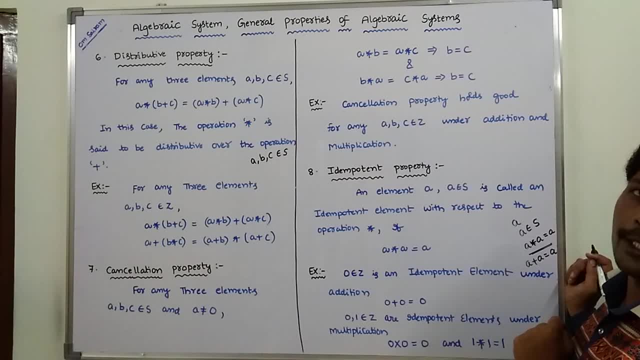 Z, So under the addition operation. So here element is 0. This element is added with the same element, Then we are getting the result is also 0. Then the idempotent property is satisfied under the operation addition. Okay, Next another example. 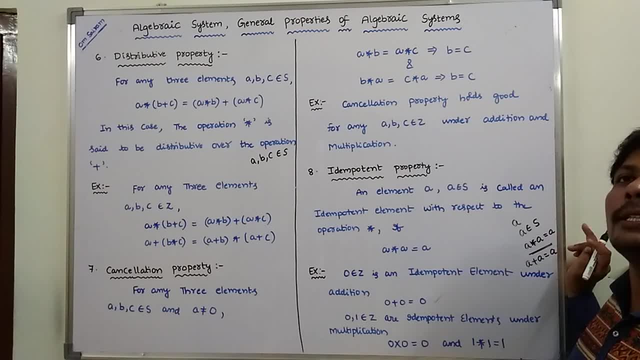 So we are taking two elements, 0 and 1, from the non-empty set Z, Okay, Under the operation multiplication. Okay, So 0 is multiplied with 0. We are getting. the result is also 0.. Next, 1 is multiplied with 1.. 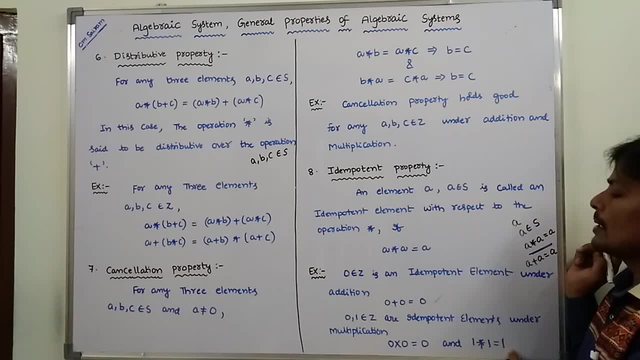 We are getting the result also 1.. Okay, So both are satisfies, the idempotent property. So then, So 0 and 1 elements are called as idempotent elements Under the operation multiplication on the non-empty set Z. Okay. 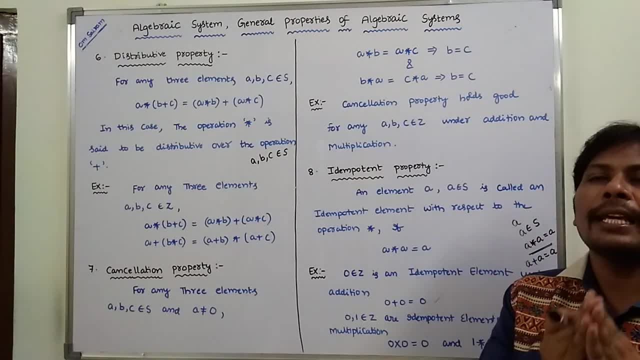 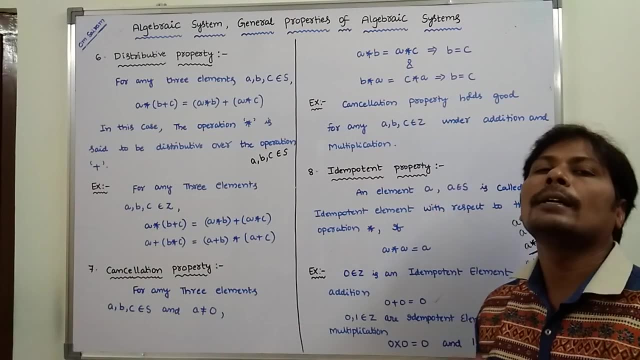 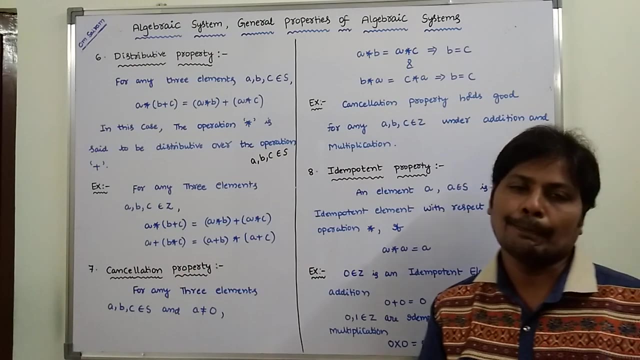 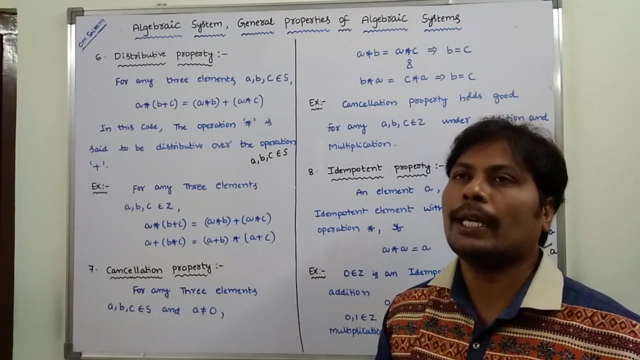 We are taking one element. This element is added or multiplied with the same element. The result is also the same element. So that is, property is called as idempotent property. Okay, So these are the properties of algebraic. Okay, So what are the properties of algebraic system that we are discussing?